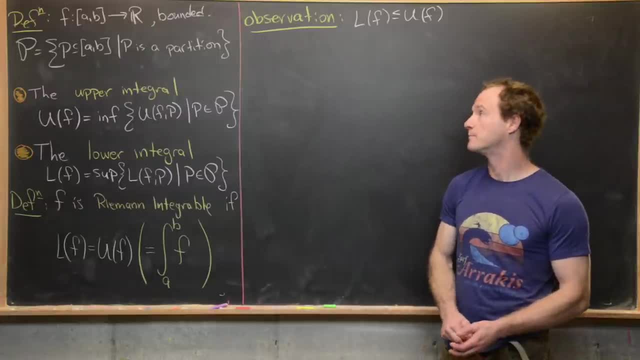 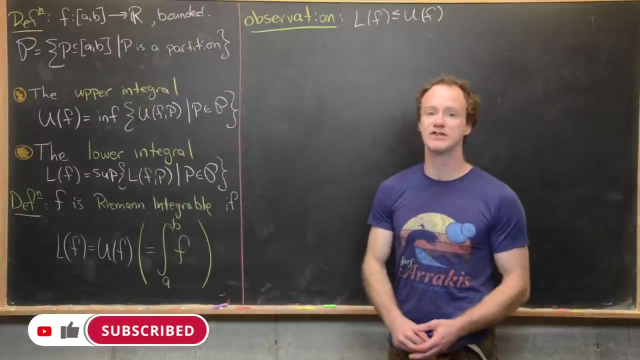 Now we're finally ready to look at the definition of integrability. So let's get to it. So let's say we've got a bounded function f from an interval a, b to r, and then we set this thing, script p equal to the set of all partitions of a- b. Then we're going to define two things: the upper, 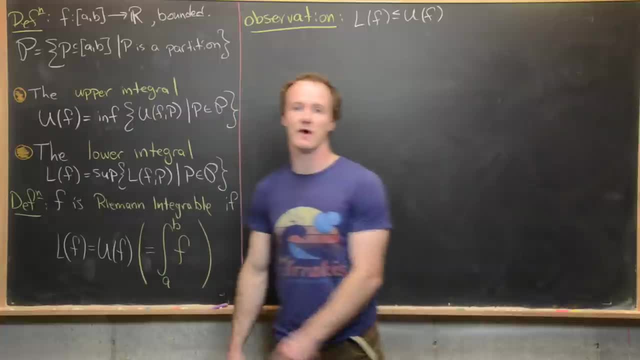 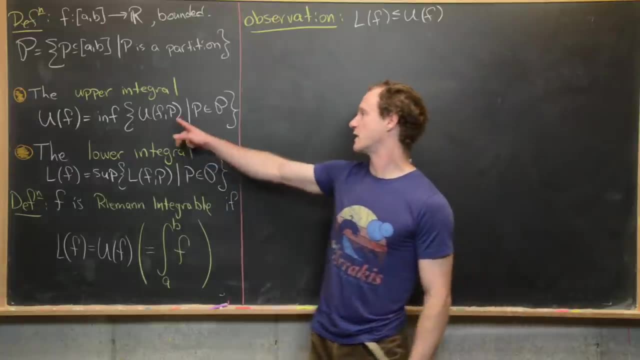 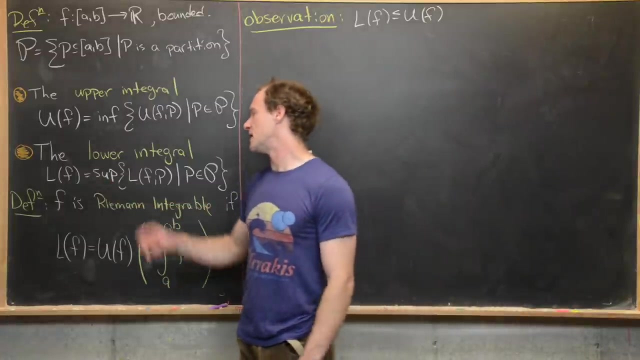 integral and the lower integral. So the upper integral of f, on this interval, is the infimum of all upper sums, as we let this partition range over all partitions of a, b. And then the lower integral is going to be the supremum of all of these lower sums as, again, we let this partition 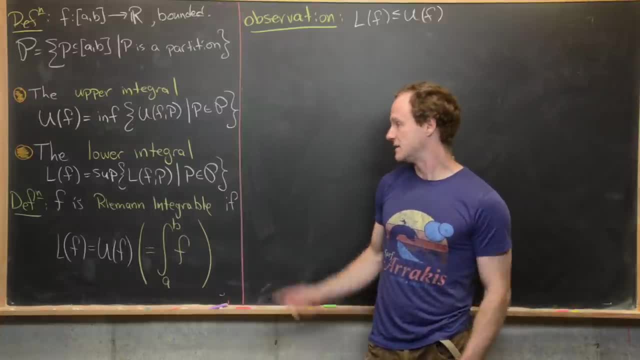 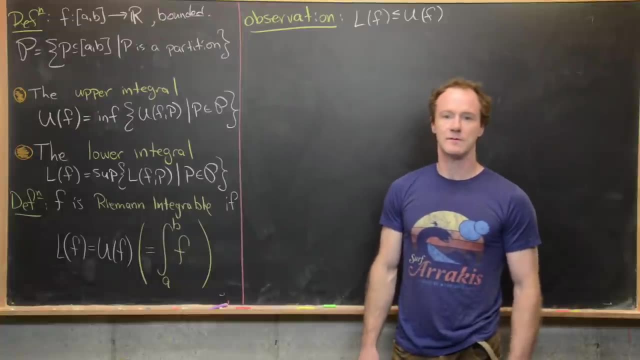 range over all partitions of a- b. Finally, we say that f is Riemann integrable if the lower integral is equal to the upper integral, And in that case we give it a new notation, which is the set of all partitions of a- b. So we're going to define two things: the upper, 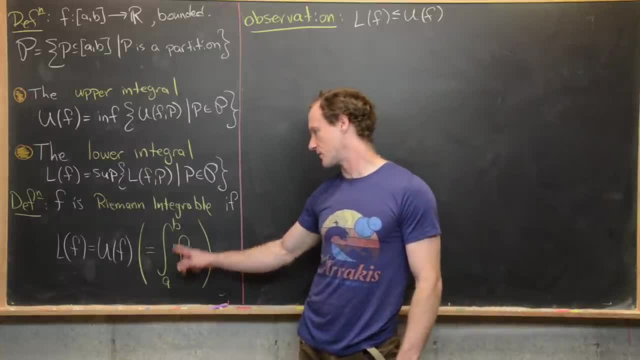 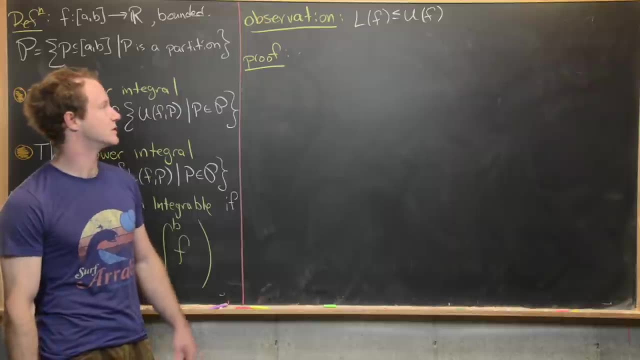 integral and the lower integral, which is probably familiar from calculus. So this is the integral from a to b of f. We're going to start by proving a pretty simple observation, but I think this is important to see the kind of tools that we'll use. So we're going to prove. 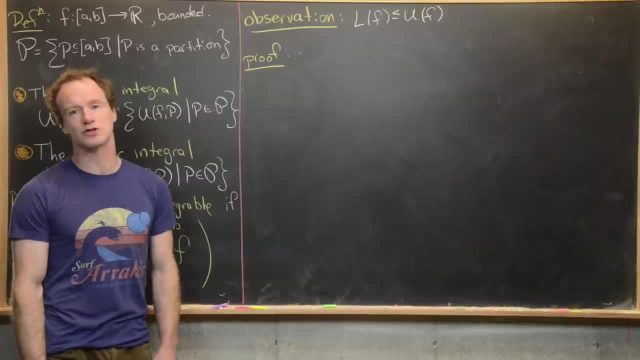 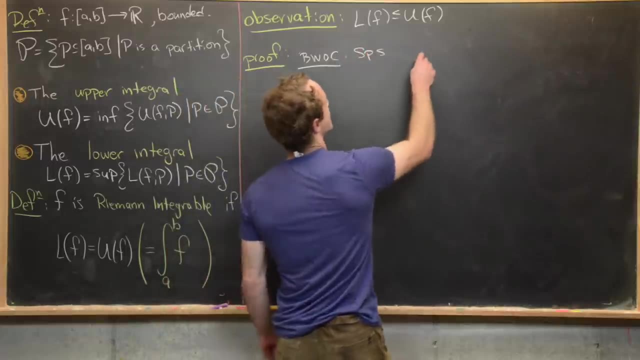 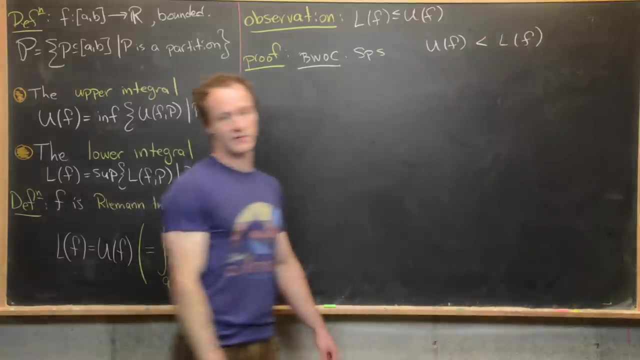 that the lower integral of f is always less than or equal to the upper integral of f. We're going to do this by way of contradiction, So in other words, we're going to suppose that the upper integral of f is strictly less than the lower integral of f. 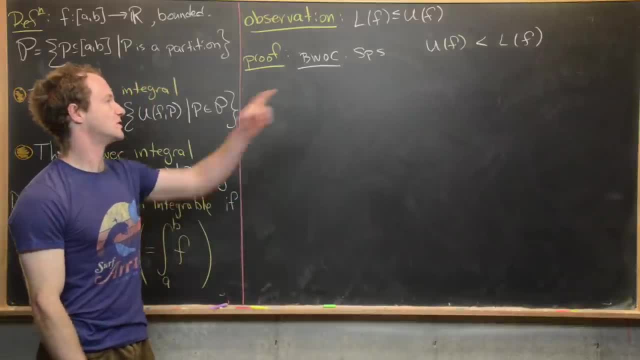 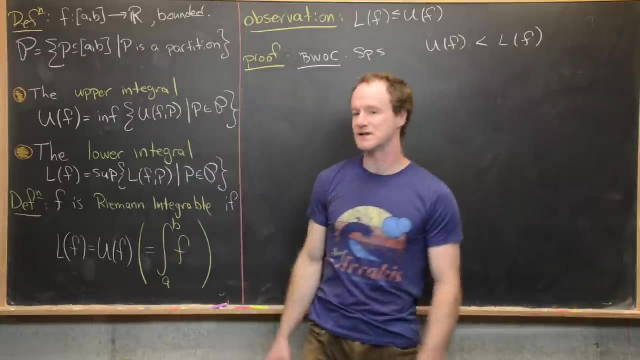 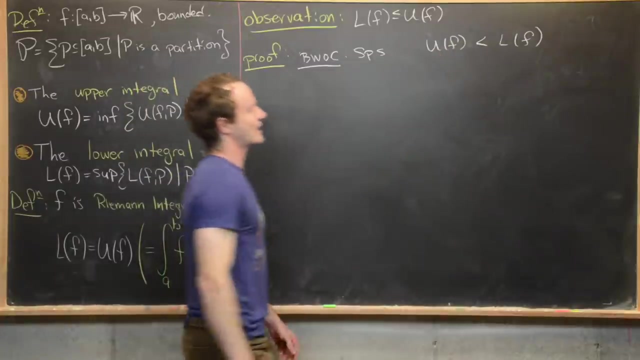 And then see that something goes wrong there. Okay, good, So notice that the upper integral of f, that is going to be the infimum of all of these upper sums. So I want to use the fact that since u of f is strictly less than l of f, there exists a partition p. maybe we'll 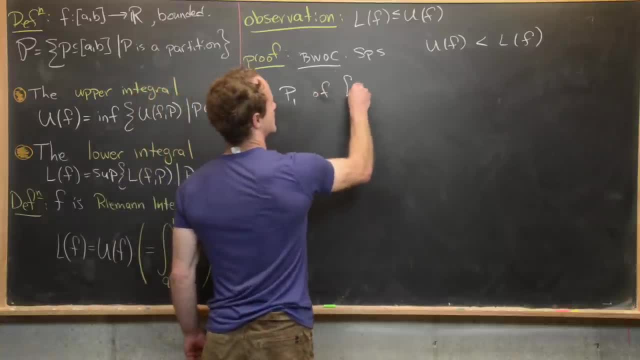 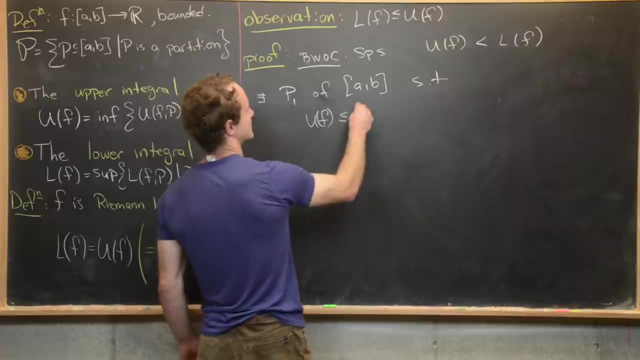 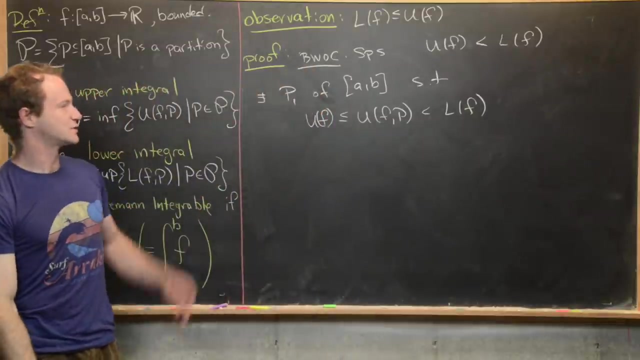 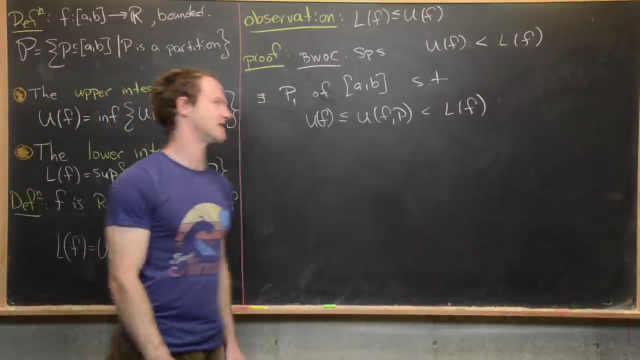 call it p1 of a- b, Such that the following is true: We have: u of f is less than or equal to u f comma p, which is strictly less than l of f. So in other words, we can find a partition where that upper sum of the partition fits in between this u f and this l f. And so why can we do? 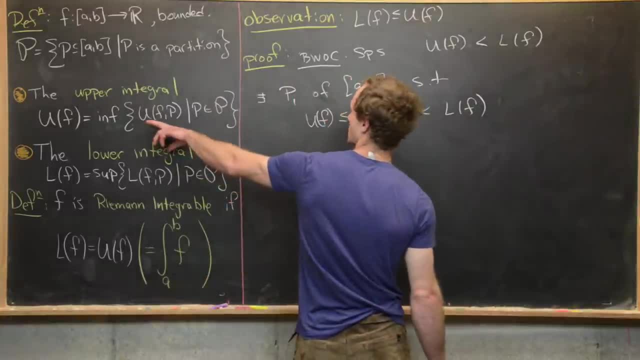 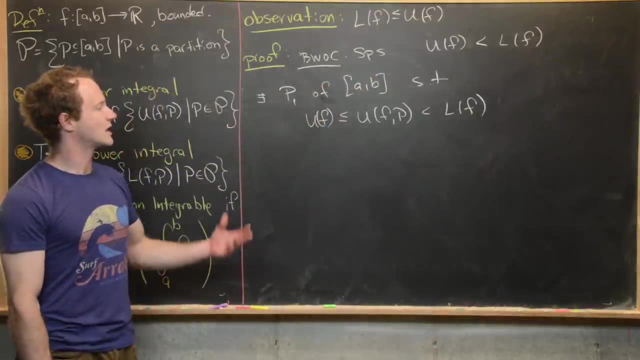 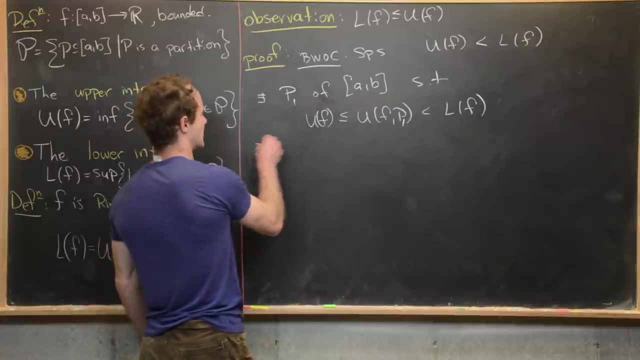 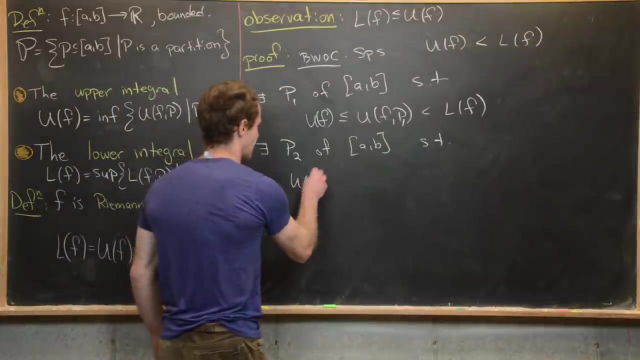 that. So if this were not possible, then we would contradict the definition of the infimum which is built into this upper. Okay, now we're going to do the same kind of thing, but we're going to do it with l of f. So let's say here that there also exists some partition p2 of a- b, such that u of f is less. 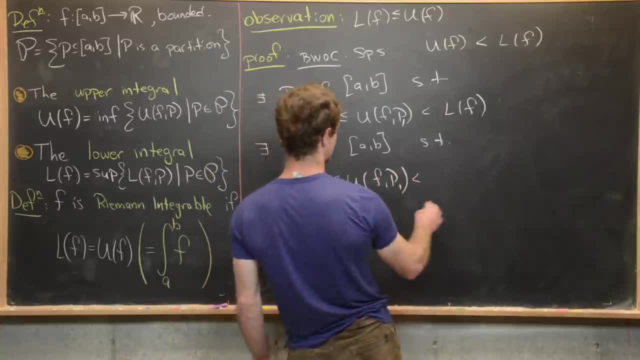 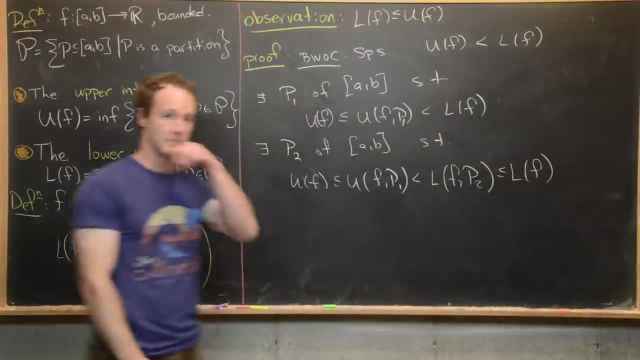 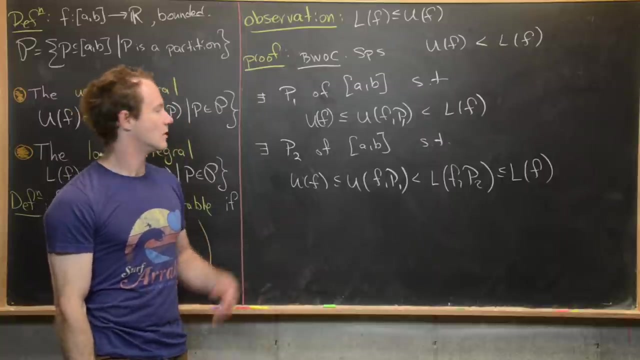 than or equal to u f p1, which is strictly less than l f p2, which is less than or equal to l of f. And again, We just need to simplify the definition of this lower integral via the supremum. So if we could not find such a partition, then this lower thing would not have been a supremum. 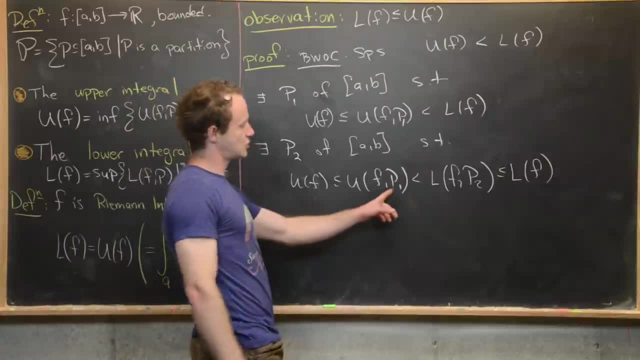 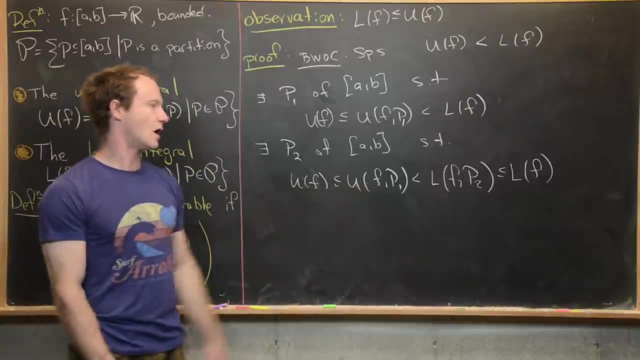 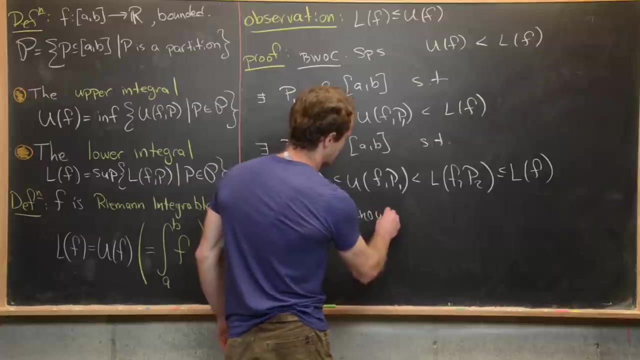 Okay, Great. So now let's see what we've got. We've got two partitions, p1 and p2, where the upper sum over one partition is smaller than the lower sum over the other partition. But we know for a fact, proven in the last video, that the lower sum of f over a partition p2 is always less than or equal. 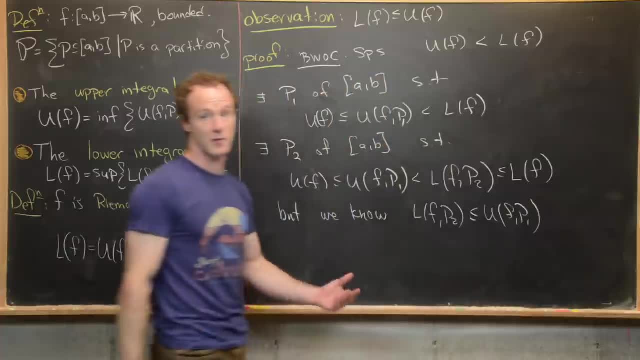 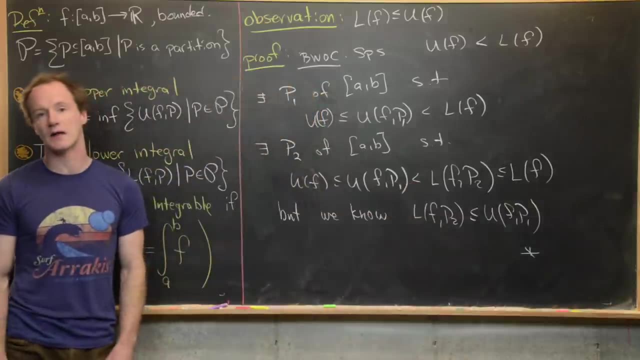 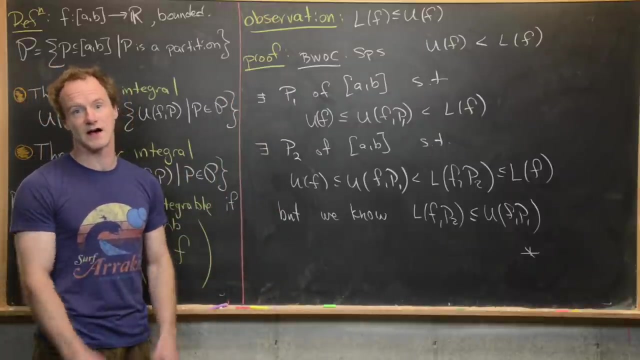 to the upper sum of f over any other partition. But that provides us with our contradiction, because this inequality and this inequality are not compatible. Okay, great, so let's maybe get rid of this, and then we're going to prove a nice theorem that classifies when a function is. 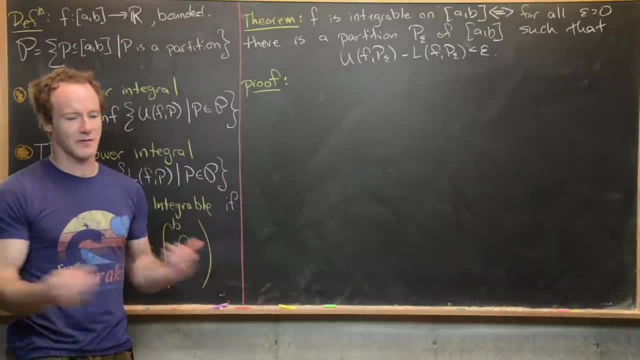 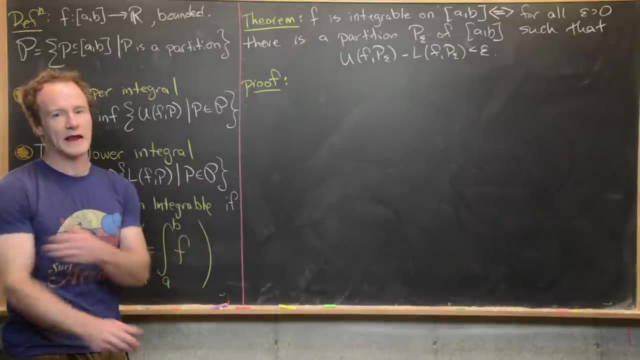 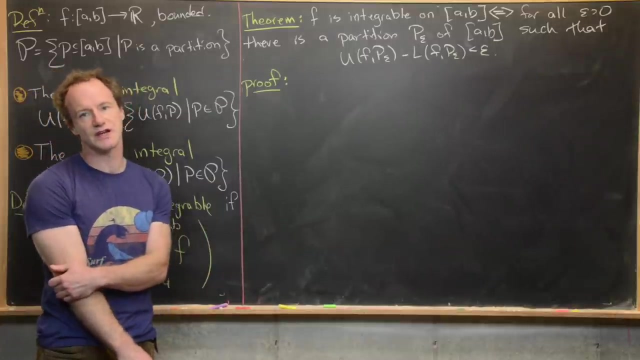 integrable. So, just like with many definitions in mathematics, often proving something via the definition is a bit tricky and what you need is some sort of more calculational approach, and often there are theorems that go and prove that this calculational approach is equivalent to the definition. That's what we've got here. So f, which is still a bounded function, 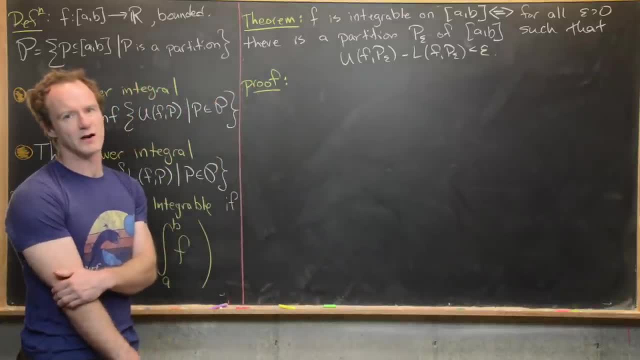 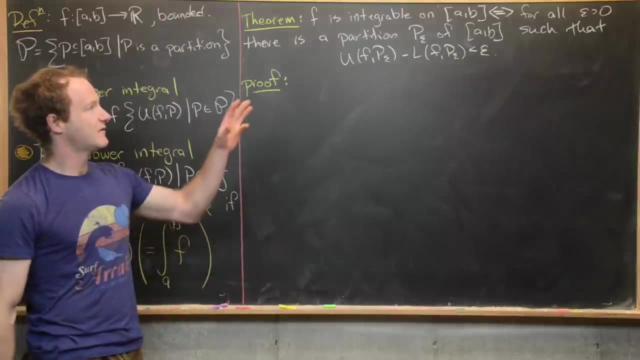 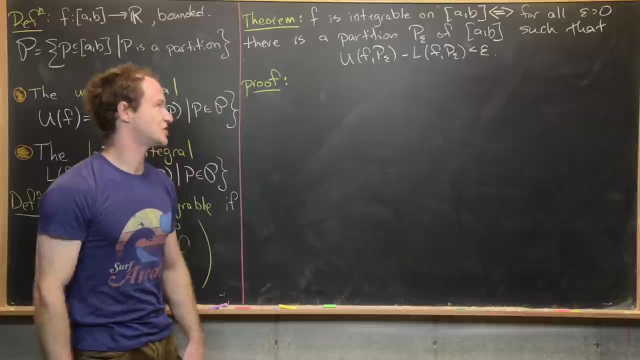 is Riemann integrable? I left off the word Riemann, but anytime we say integrable, for the time being it will be Riemann. integrable On the interval a- b, if, and only if, for all epsilon bigger than zero there is a partition p epsilon of a- b, such that the upper sum of f on that partition 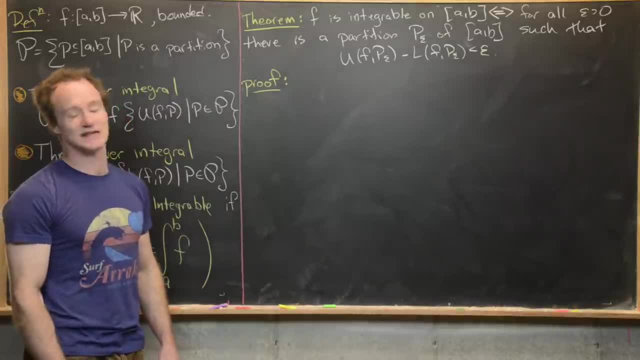 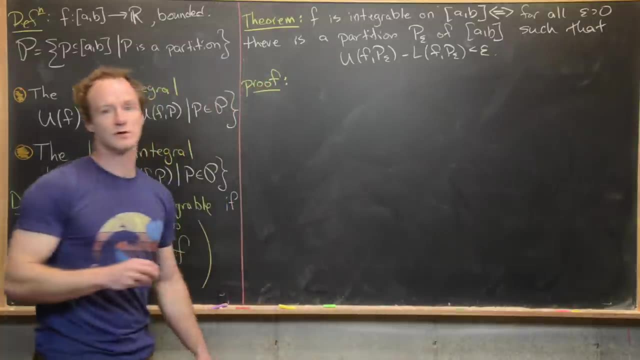 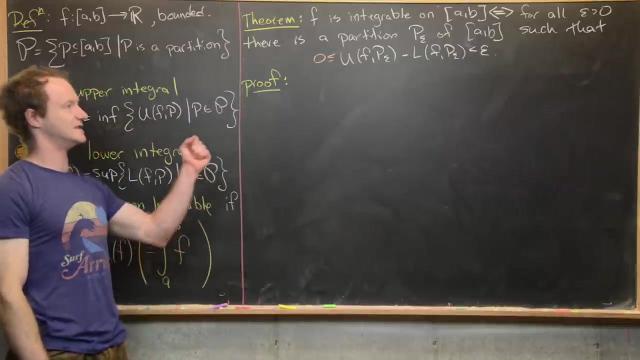 minus the lower sum of f on that partition is less than epsilon. Now maybe I want to point out real quick that the upper sum is always bigger than or equal to the lower sum, so we know that this is going to be always bigger. So this is bound between zero and epsilon, But since epsilon can be made as small as we want, 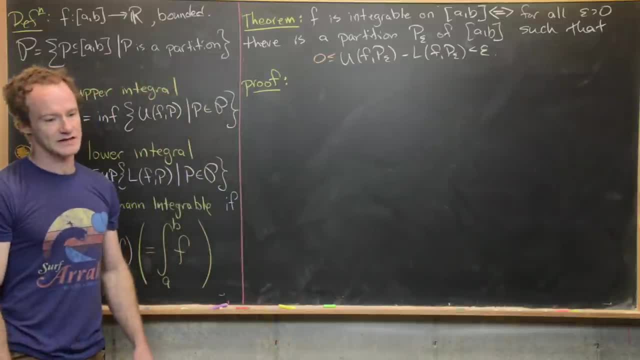 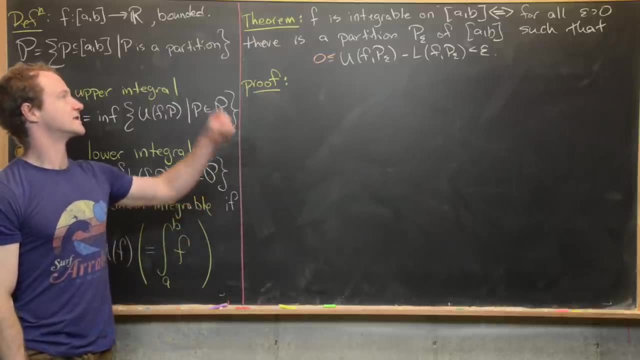 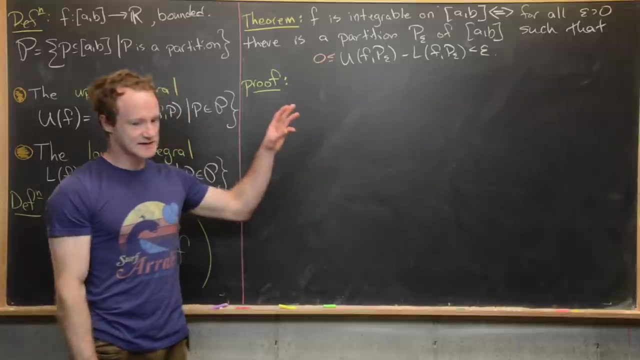 that means these two quantities can be made as close together as we want. So notice: the right hand side of this if and only if statement is very calculational, whereas the left hand side is built out of this definition that we have over here. Okay, so let's maybe get to the proof. So, since this is an if and only if statement, we need to 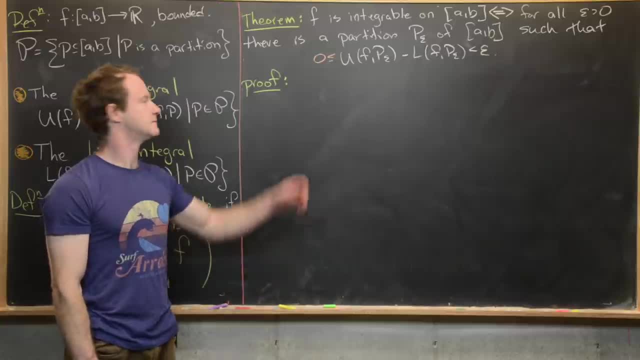 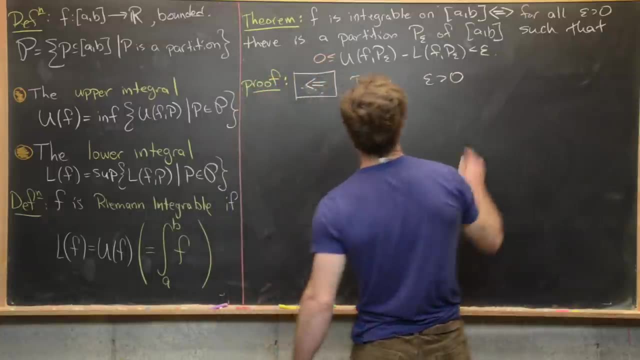 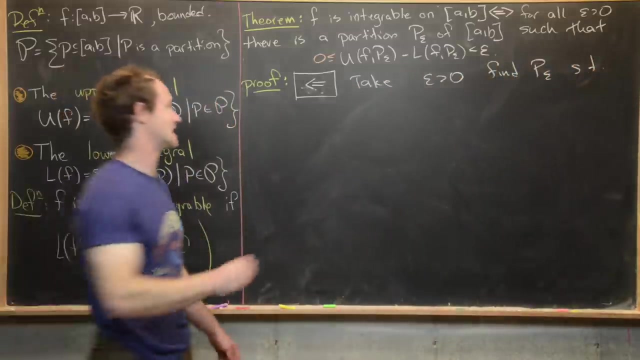 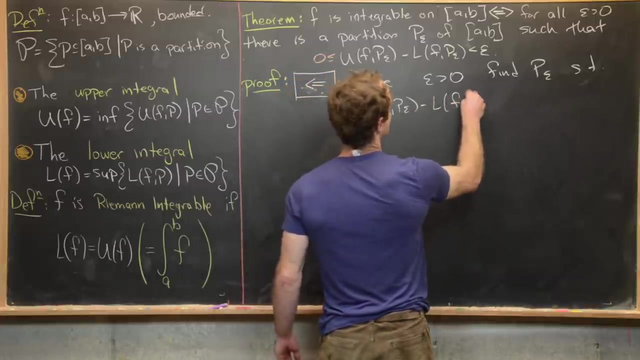 do two directions. So let's start with this, The reverse direction. So we're going to begin by taking any epsilon bigger than zero and then finding our partition p epsilon, such that this inequality is satisfied. So we've got: zero is less than or equal to u f p epsilon minus l f p epsilon, which is less than epsilon Great. So again we're. 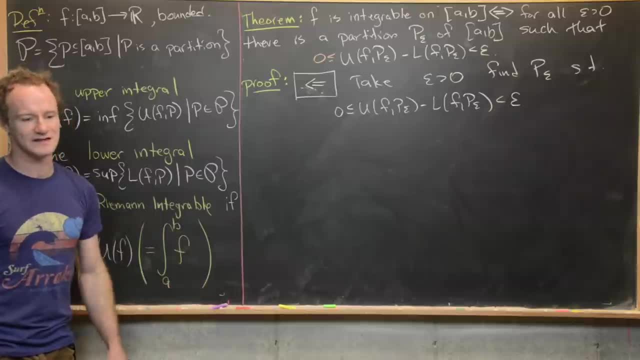 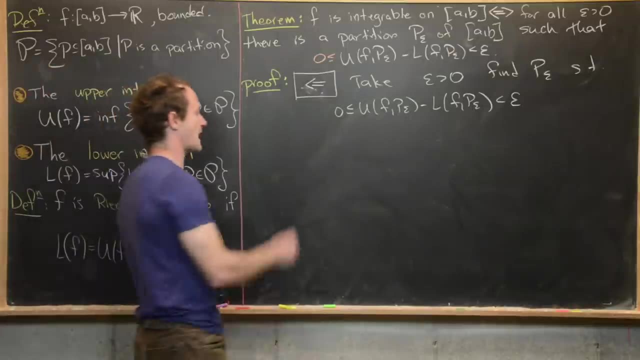 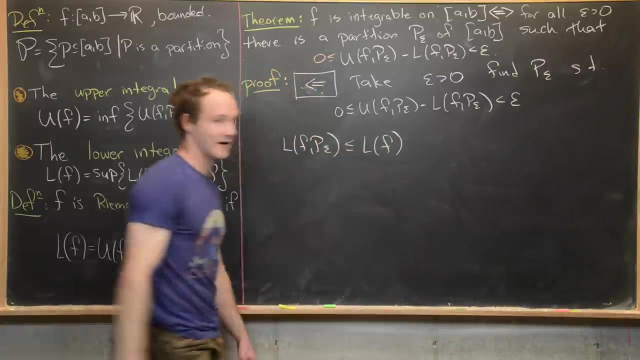 working backwards or the reverse direction. So we can assume that this kind of thing is possible. Now we're going to use the following string of inequalities, which is always true, And that goes like this: l, f, p, epsilon is always going to be less than or equal to l of f, So in other words, the lower sum is always less than or equal. 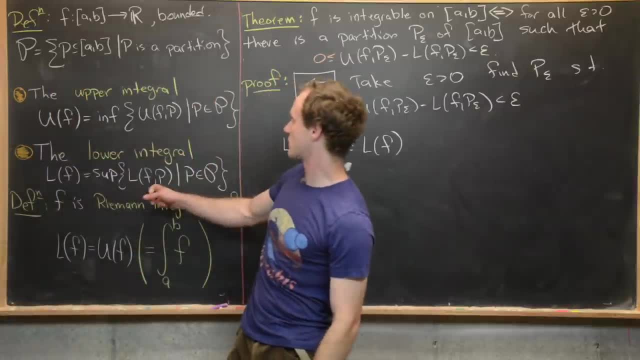 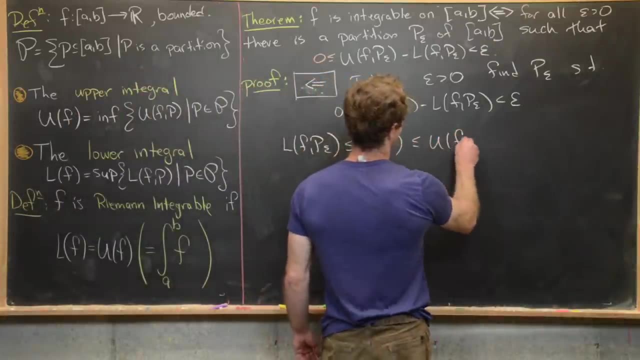 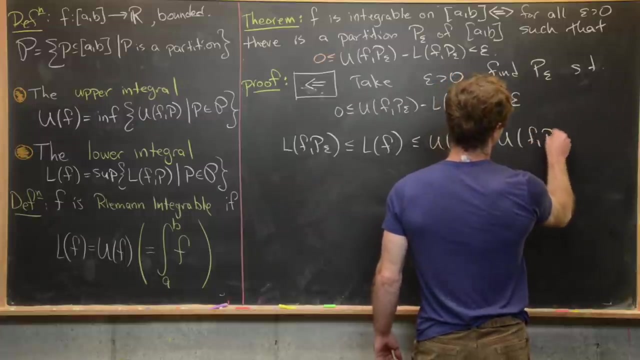 to the lower integral. That's because this lower integral is the supremum of all such lower sums. But now that's less than or equal to u f p epsilon minus l f p epsilon. So we're going to use this string of inequalities Again, because the upper integral is always less than or equal to the upper 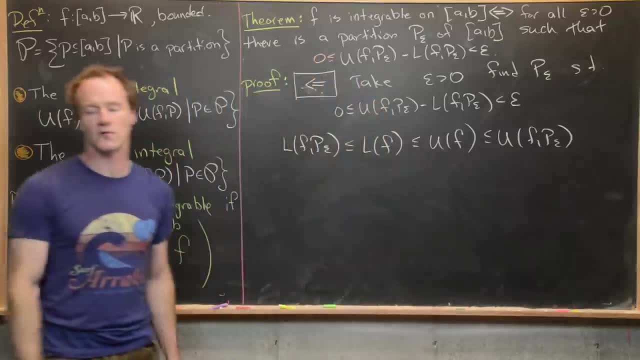 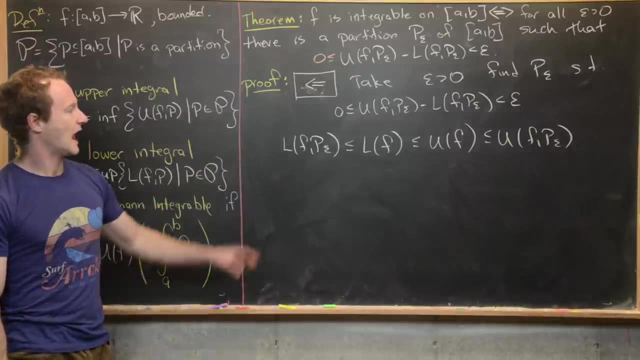 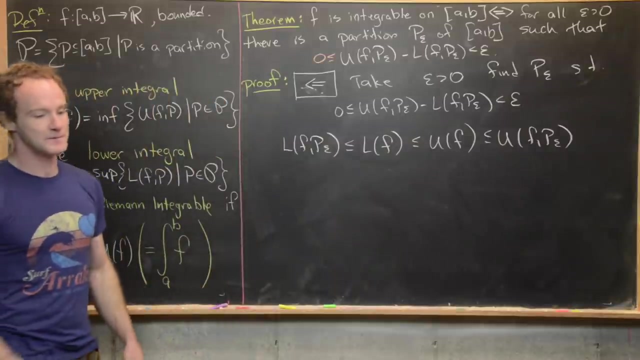 sum, given that the upper integral is the infimum over all such possible upper sums. But now we can look at this string of inequalities And use the fact that these two are close together to force two close together. In other words, we have the following setup: We have U of F. 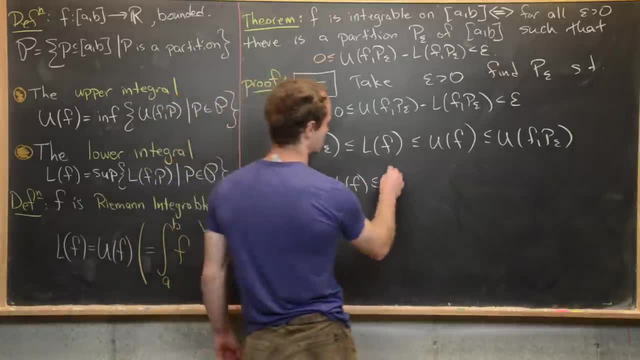 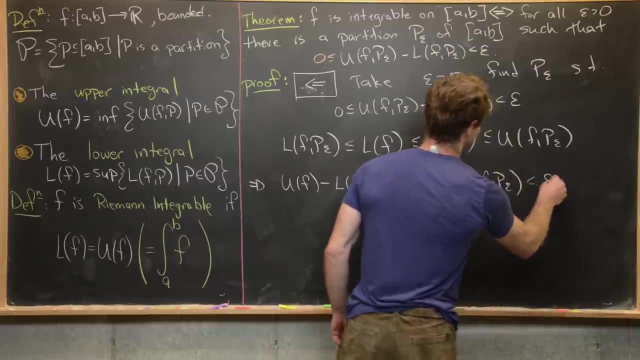 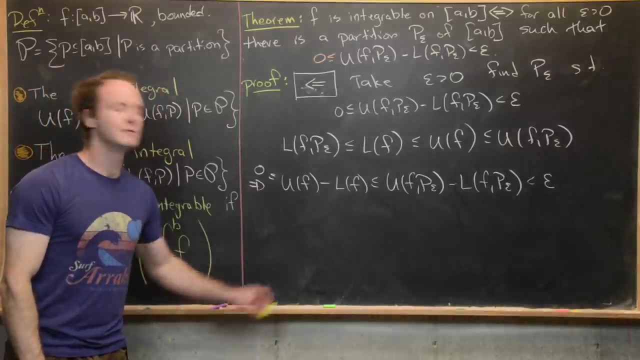 minus L of F is less than or equal to U F P epsilon minus L F P epsilon. but that's less than epsilon. And then I guess I should maybe say over here that all of this is bigger than or equal to 0.. So let's see what we've got going on. 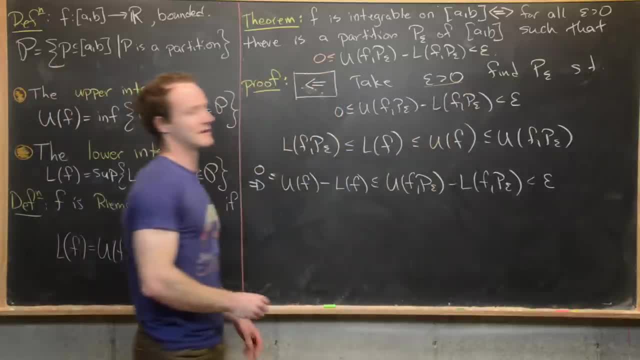 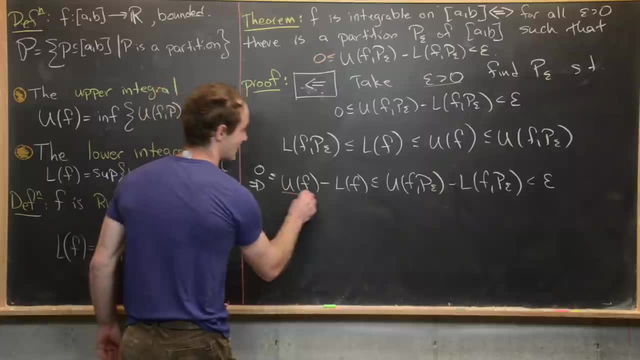 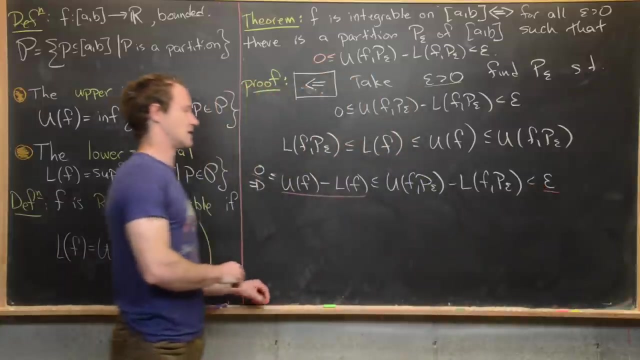 here We've got this arbitrary epsilon bigger than zero and after taking this arbitrary epsilon bigger than zero, we have shown that the difference of the upper integral and the lower integral is bound between zero and epsilon. So in other words, we can make this difference between the upper integral and lower. 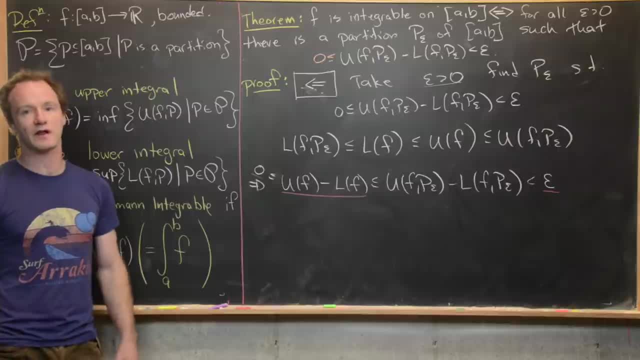 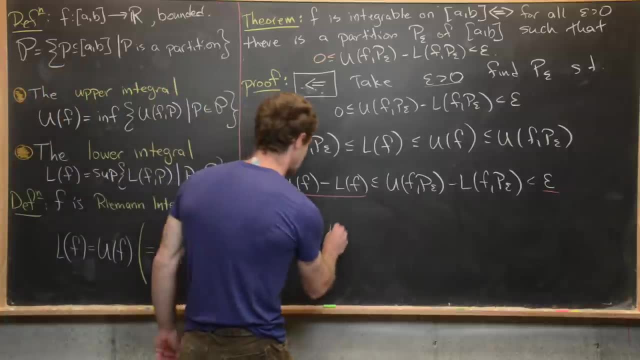 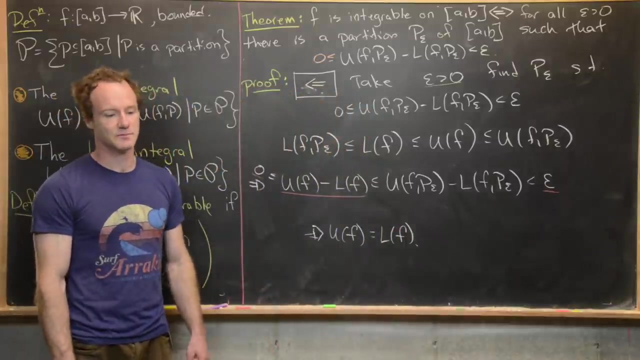 integral as small as we want. They are arbitrarily close together, but from one of the maybe first theorems that we proved in the whole class that tells us that these two numbers, uf and lf, are the same. And that finishes this reverse direction. Okay, let's maybe do the forward. 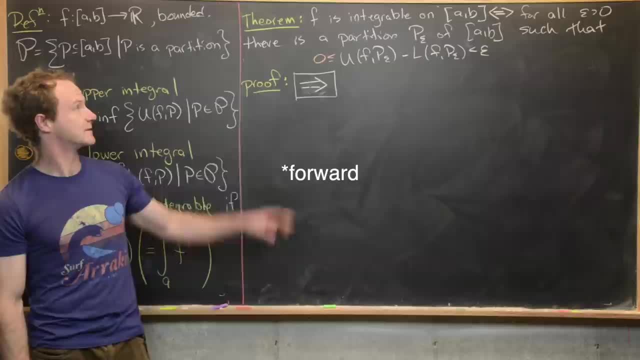 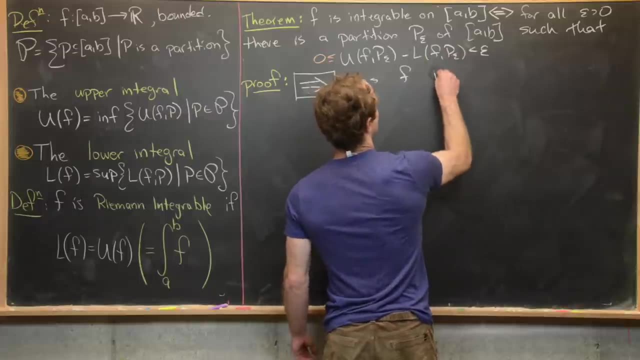 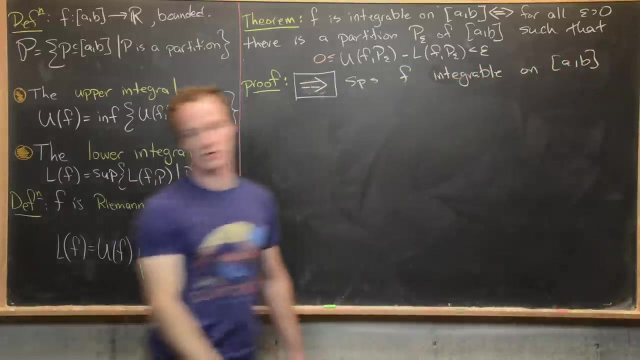 direction now. Now we're ready for this reverse direction. So we want to suppose that f is bounded and Riemann integrable. So I'll just say integrable on our interval. a, b, Good, And then next we also want to be given some arbitrary epsilon. 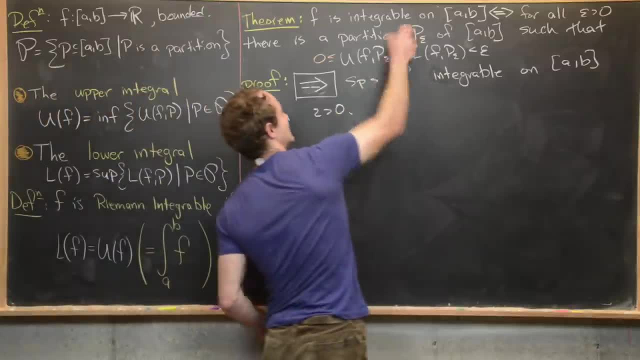 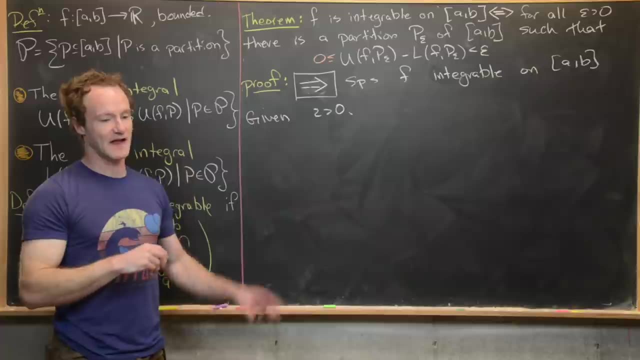 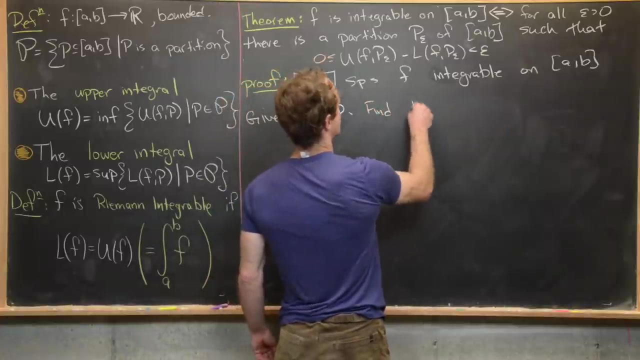 bigger than zero, And then our goal is to find this partition that makes this inequality true. Okay, so we want to do two things first, and that is find a partition related to the upper integral and the lower integral. So let's first find p1,. upper integral and then find p2, upper integral. So let's find p1, upper integral and then find p2, upper integral. So let's first find p1, upper integral and then find p2, upper integral. 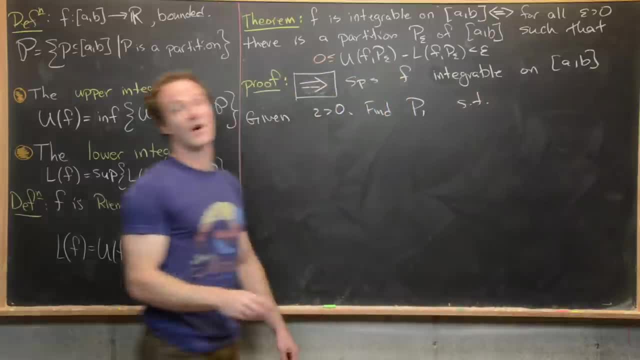 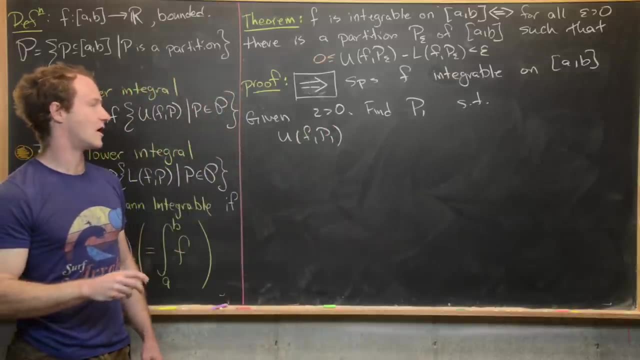 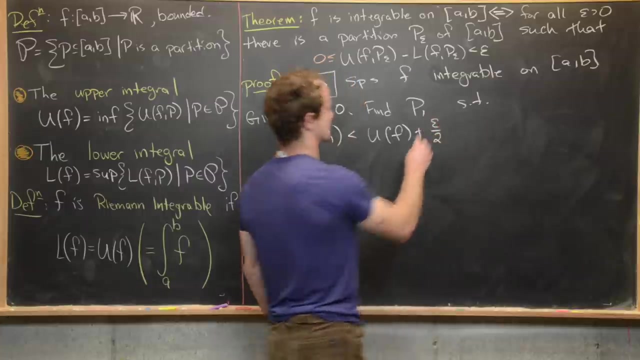 partition of a- b such that the following inequality is true: We have uf- p1.. In other words, that upper sum of f on p1 is less than uf plus epsilon over 2.. So let's maybe talk our way through why we can do that. Well, if that were not possible, 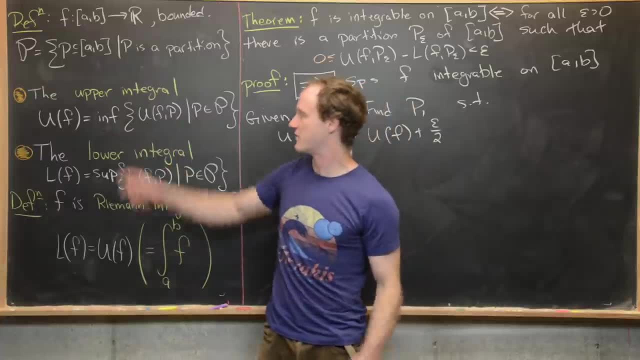 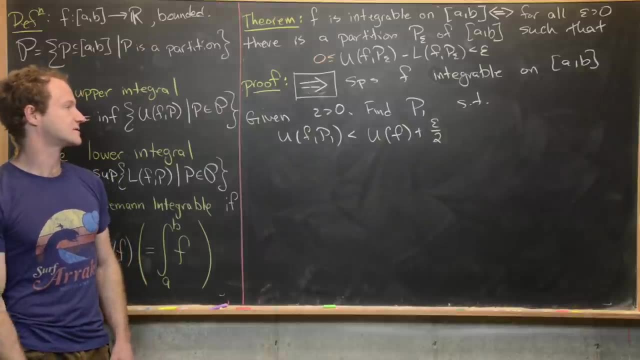 that would contradict the definition of uf by the infimum, And actually this kind of construction was something really familiar that we did at the very, very beginning of the class. Okay, great, And then next we want to find a partition p2,. 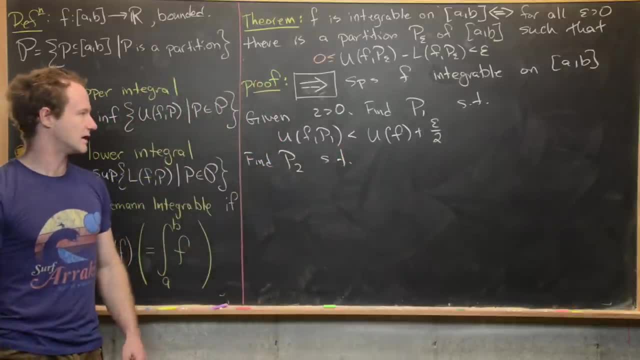 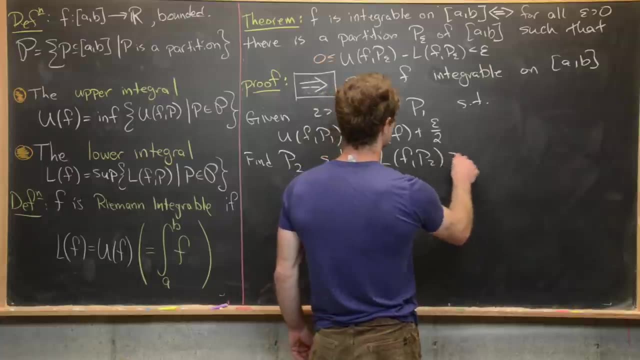 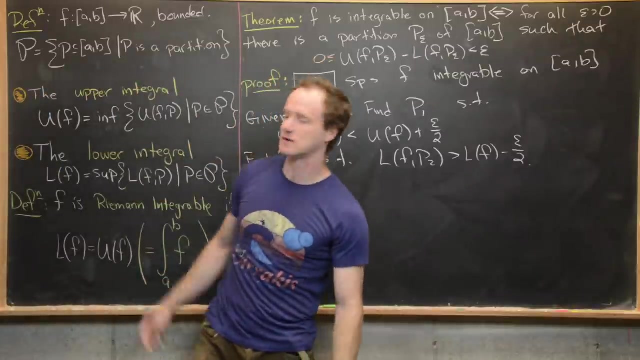 such that we've got a similar but different inequality for the lower sum and lower integral, And in this case we want lf p2 to be bigger than lf minus epsilon over 2.. And again, that's by the definition of the supremum. 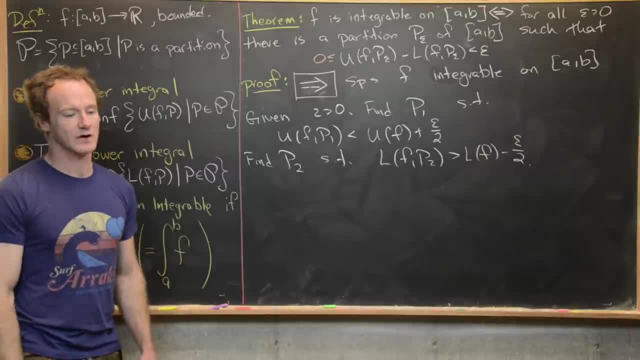 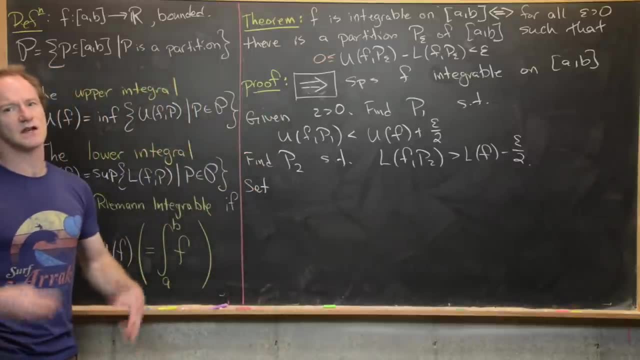 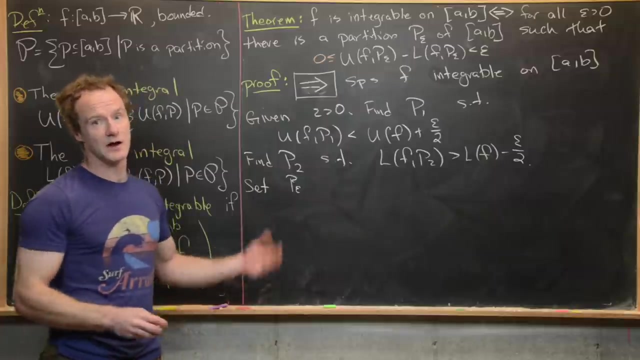 Or the least upper bound. Okay, great. Now what we want to do is form a partition out of p1 and p2.. And this is going to be the so-called common refinement, And we'll call that common refinement. p sub epsilon. So that'll be our partition, that we want. So we've got p sub epsilon equals p1. 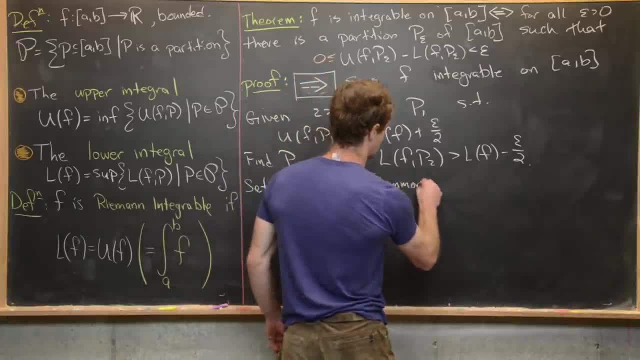 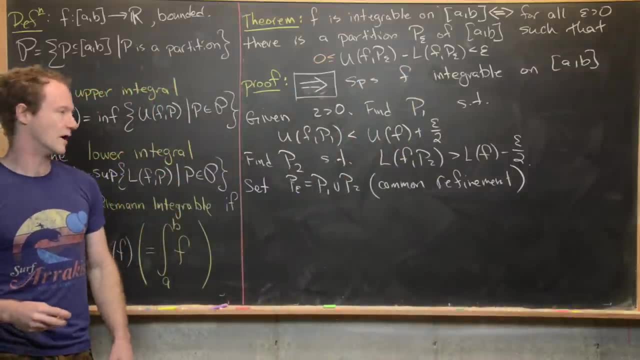 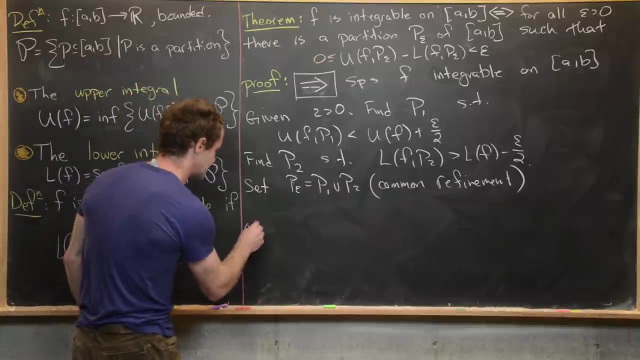 union p2.. So, like I said, this is the common refinement of p1 and p2.. Look in one of the videos if you need a reminder of what the refinement of a partition is. Now let's look at our goal thing right here. So we have: zero is less than or equal to uf p, epsilon minus lf p. 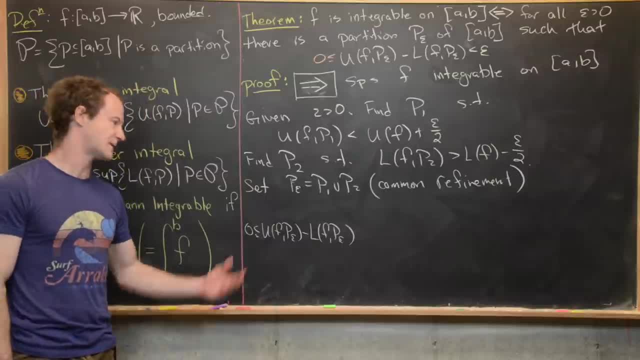 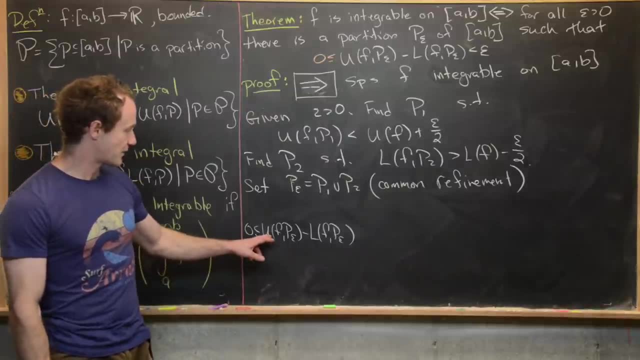 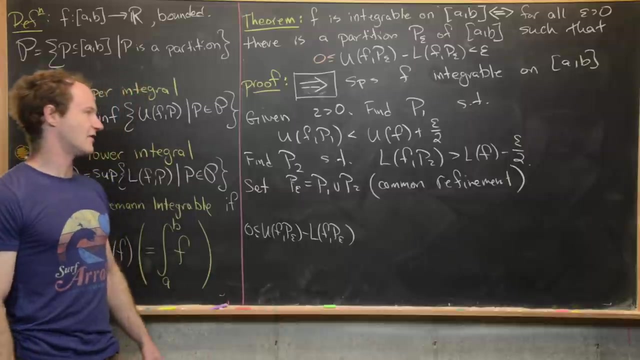 epsilon. So we know that this is going to be bigger than or equal to zero, just by the definition of the upper sum and the lower sum. But next thing that I want to do is replace uf p epsilon with this thing that is larger, And I'll replace lf- p epsilon with this thing that is smaller, But that's going to keep my 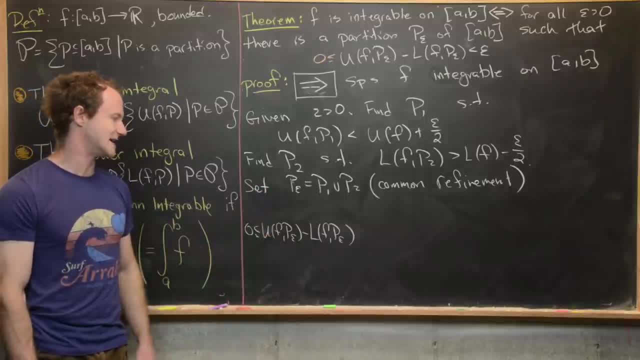 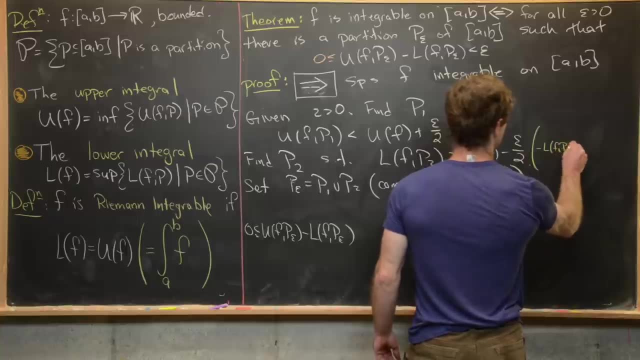 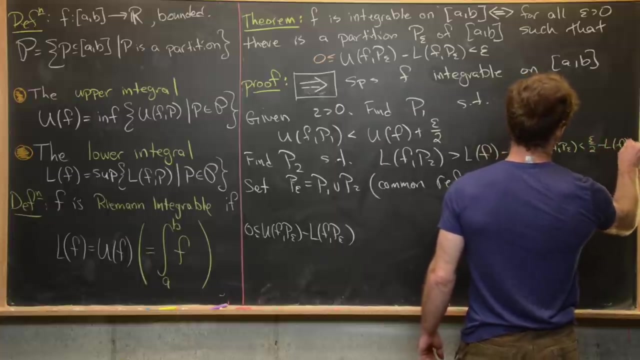 inequality going in the correct direction because I have minus lf p epsilon. So in fact I'm going to use this fact right here, that minus lf p epsilon is in fact less than epsilon over two minus l of f. Just multiplying by the minus one changes the direction. But now we can. 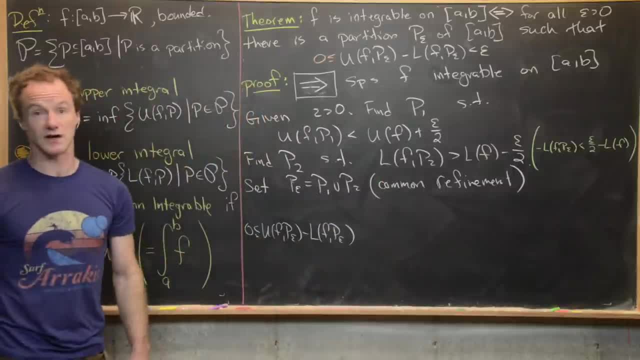 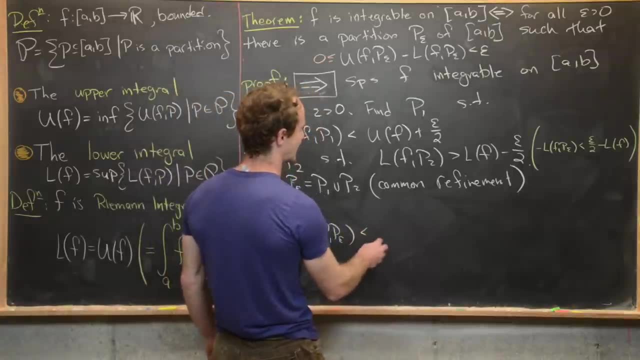 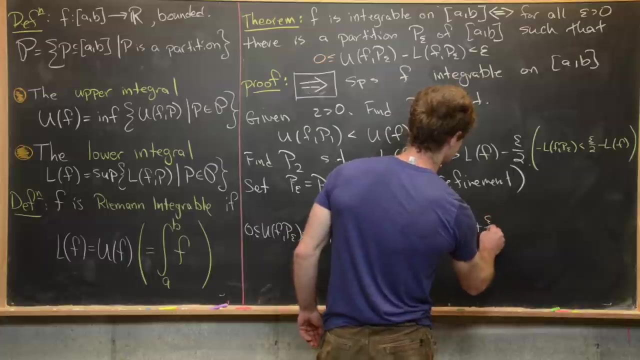 just like: essentially, add these two inequalities and we're done. So let's see what we get when we do that. So here we will get that this is strictly less than u of f minus l of f plus epsilon over two plus epsilon over two. But we know that u of f and l of f are the same because we have assumed. 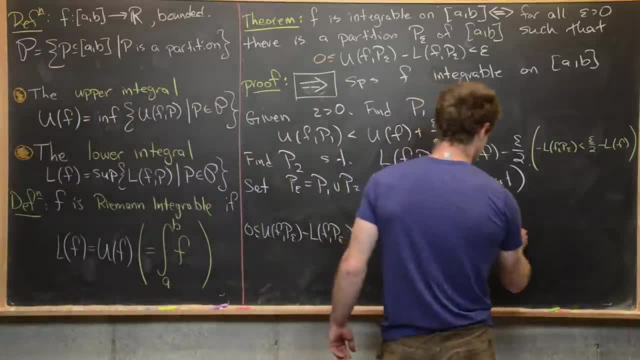 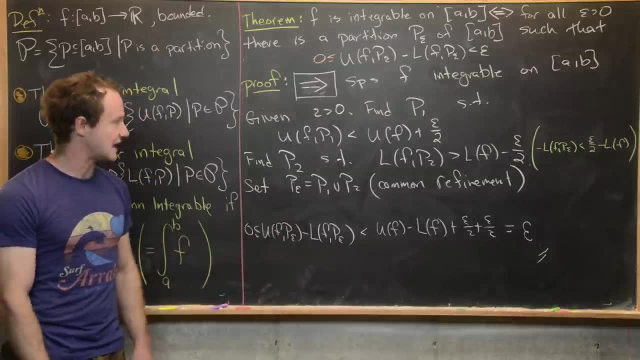 integrability of our function f. So that turns out to be epsilon over two plus epsilon over two, which is epsilon. So in the end we have our desired inequality to finish off this forward direction. Okay, let's get rid of this and we're going to do one more theorem. 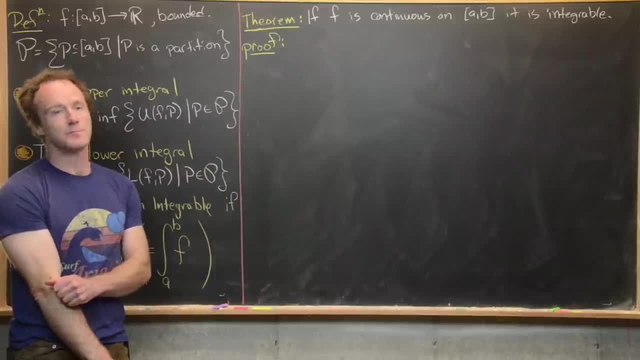 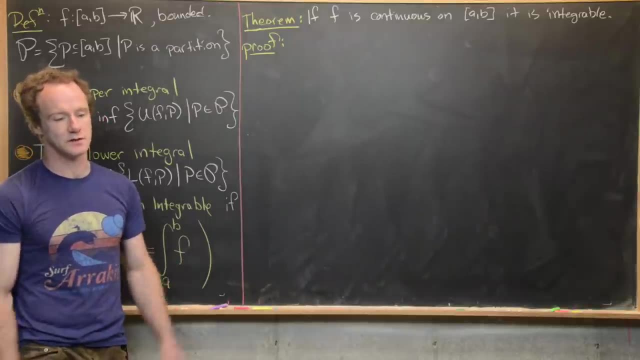 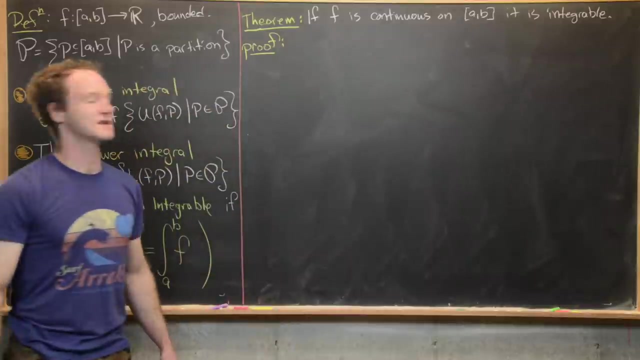 We're going to finish this video off by looking at a classic and very important theorem. So this says that if f is continuous on a closed interval, a- b, then it is integrable on this closed interval as well. So I first want to notice that continuity plus the compactness of this closed interval. 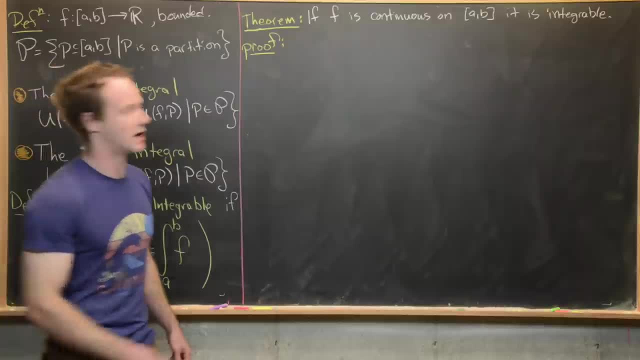 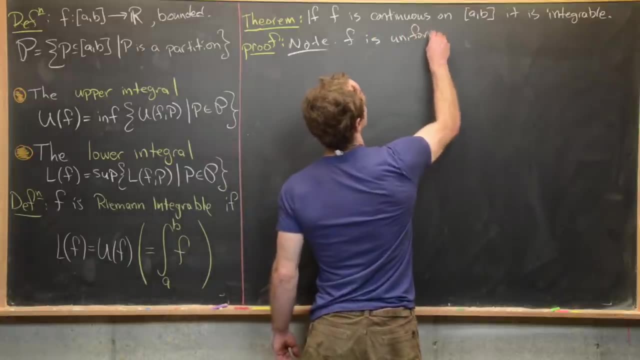 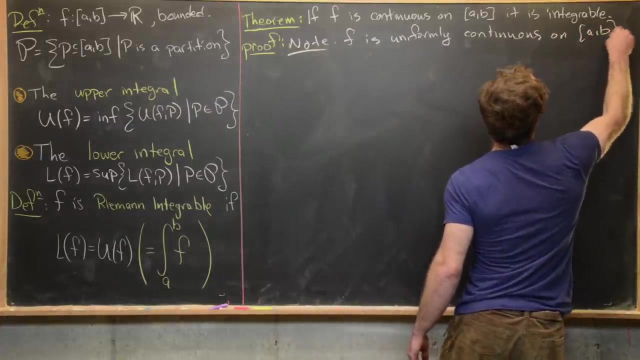 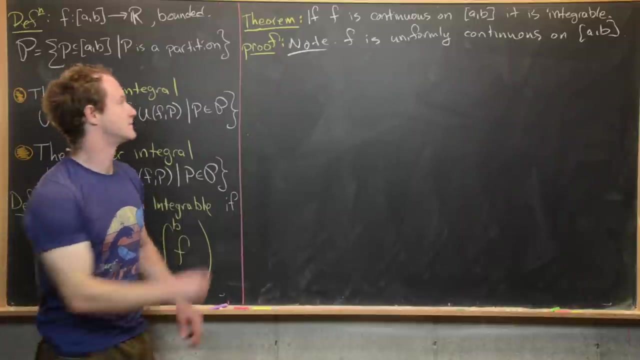 implies that f is uniformly continuous on a- b. So let's maybe notice that first. So f is uniformly continuous on our interval a- b. Again, because continuity plus compactness of the domain implies uniform continuity. Okay, so next we want to be given epsilon bigger than zero. 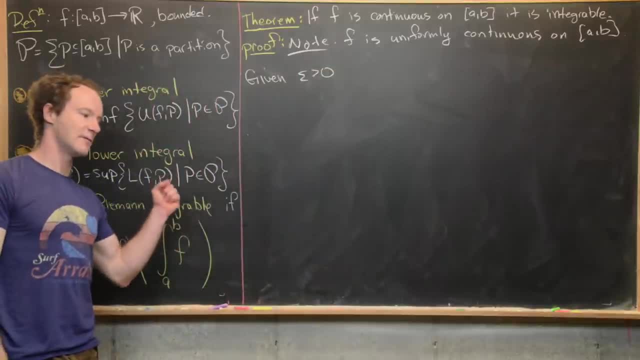 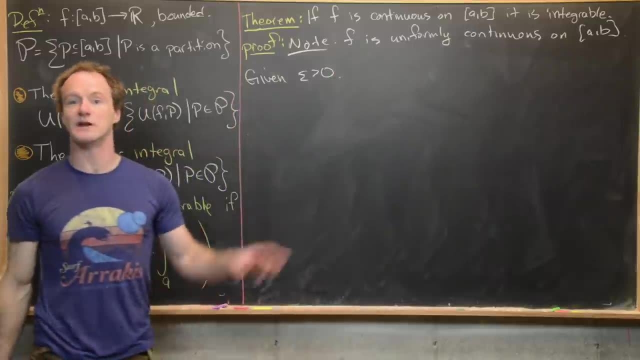 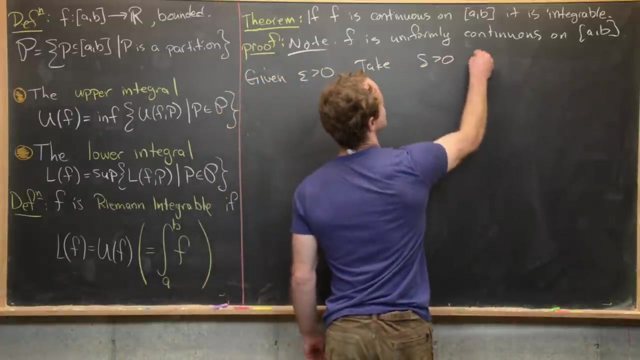 And our goal is to form a partition that makes the upper sum minus the lower sum over that partition less than epsilon. Okay, but we need to use this continuity. In fact, we want to use this uniform continuity. So let's go ahead and take delta bigger than zero, Such that if the absolute value of x minus y is less, 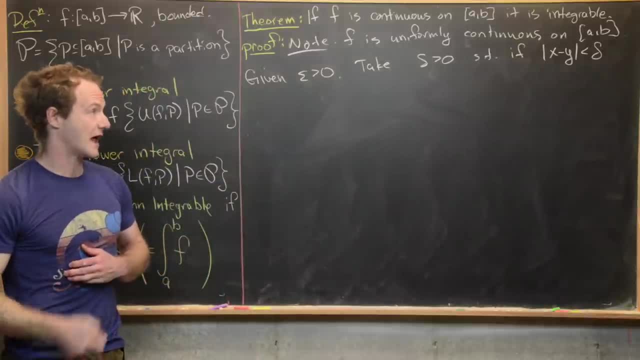 than delta where x and Y are both on the interval a- b but they're within delta of each other. we have the absolute value of x minus y is less than zero. We want toroffen delta where the absolute value of Y is by cosine todos, as I mentioned in the first när. 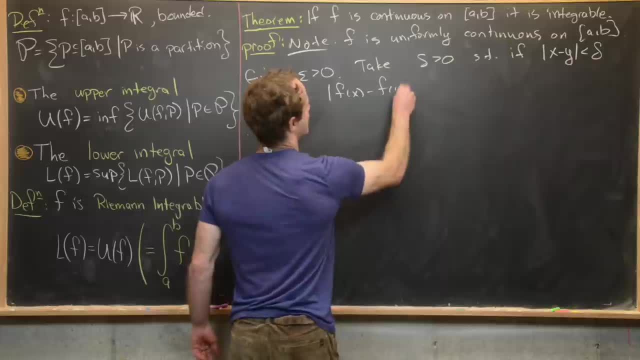 something- Page 9, 1,, 2,, 3,, 3, and 4.ama- as the inner derivative of a- b. So F1 is well, r1, not it. But again, absolute value of f, of x minus f of y is less than not just epsilon, but epsilon over b minus a. 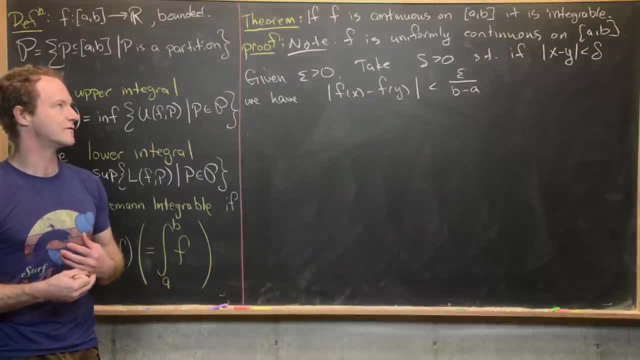 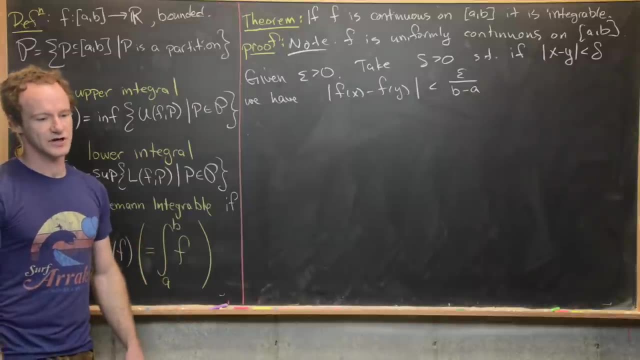 so, again, this delta is brought into existence because of the uniform continuity of f on a- b. that's why it works for all x and y within delta of each other. okay, great, now we're going to start constructing our partition. there's a bunch of ways to do this. i'm going to do this a very concrete. 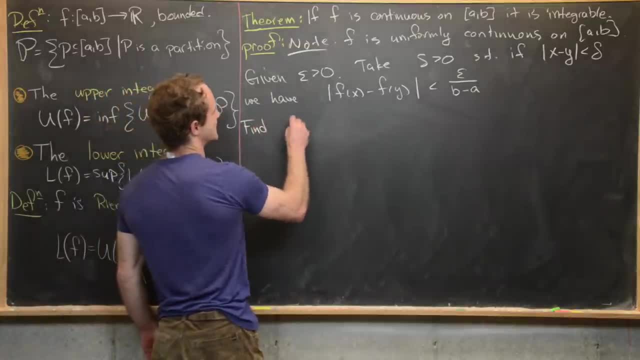 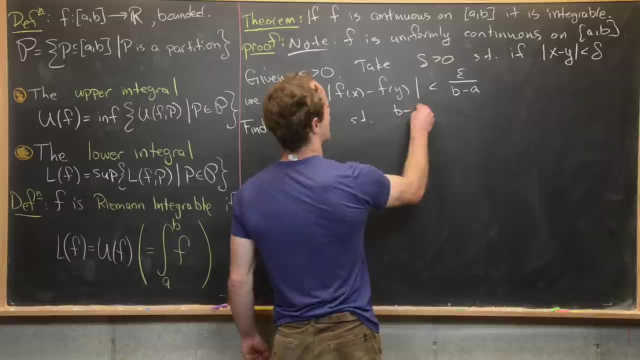 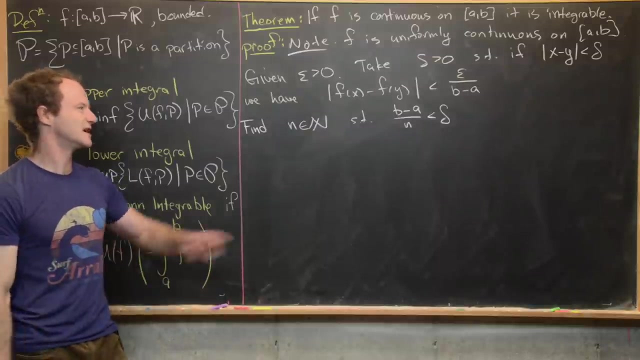 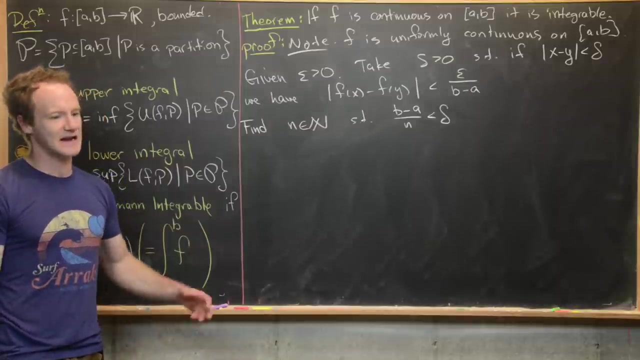 way. so let's go ahead and find some natural number, which i'll call n, such that b minus a over n is less than delta, and so that's possible by the archimedean principle, because you can maybe move this around until you get. n is bigger than some real number. but you know, you can always find 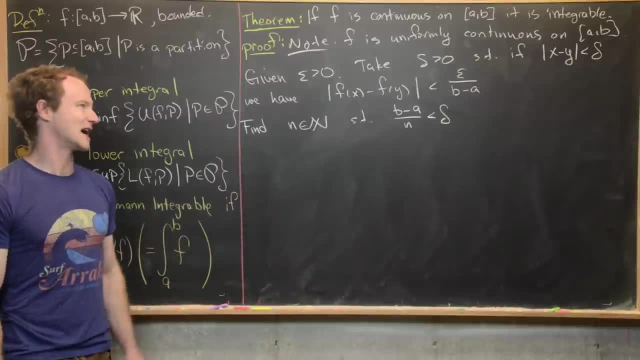 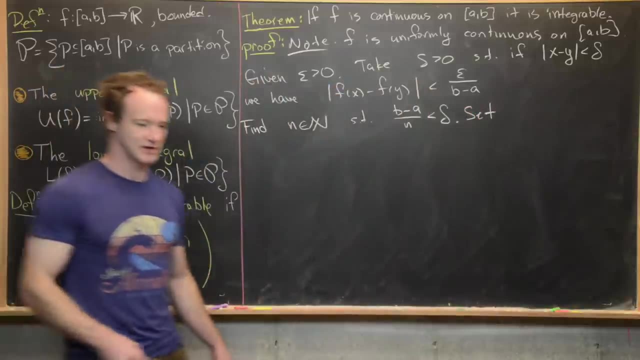 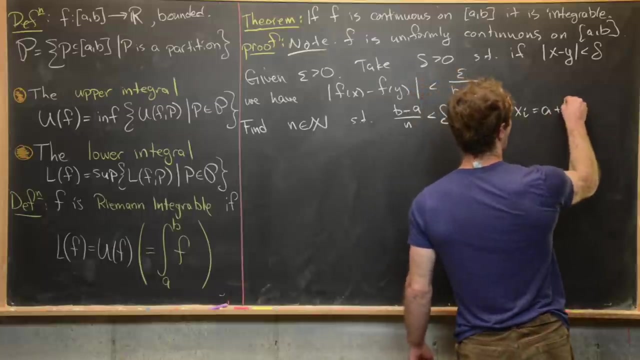 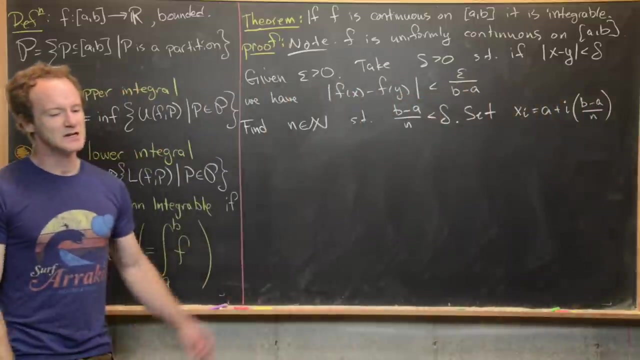 a natural number bigger than any real number. but again, this is the kind of stuff that we do all the time at this point. okay, so next we want to define the points in our partition. so i'm going to define them like this: we'll set x- i equal to a plus i times b minus a over n. good, so this is like a plus i, delta x, like 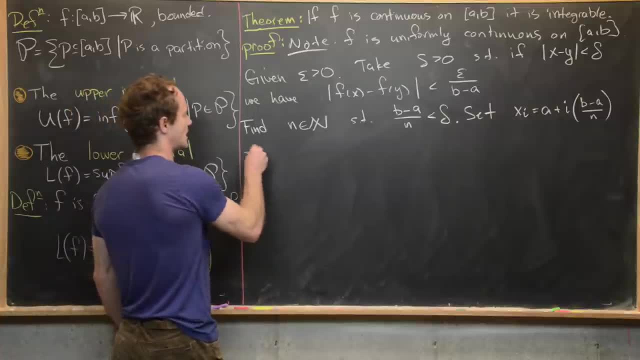 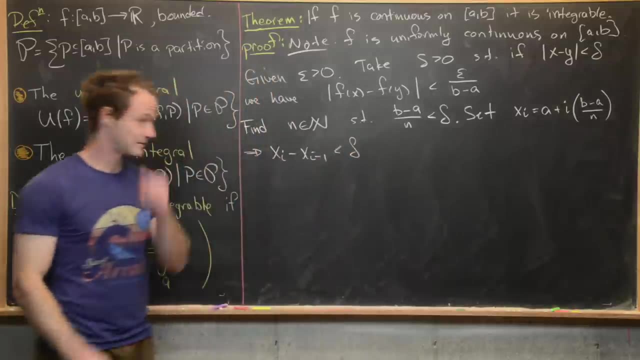 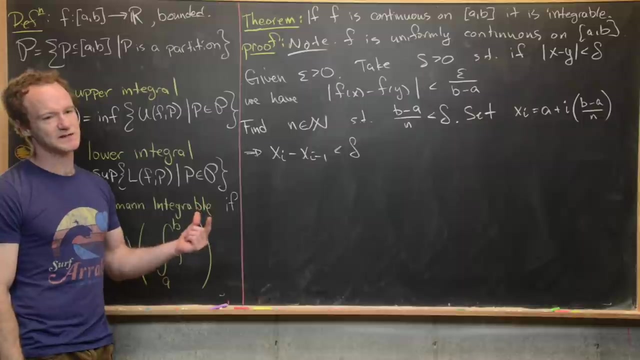 you might have seen in a calculus 2 type class. now what i want to notice here is that x i minus x, i minus b minus a over n is less than delta x. so this is like a plus i delta x, like you might not be sure of. 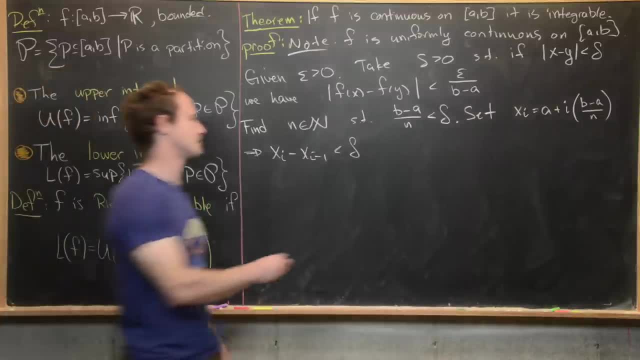 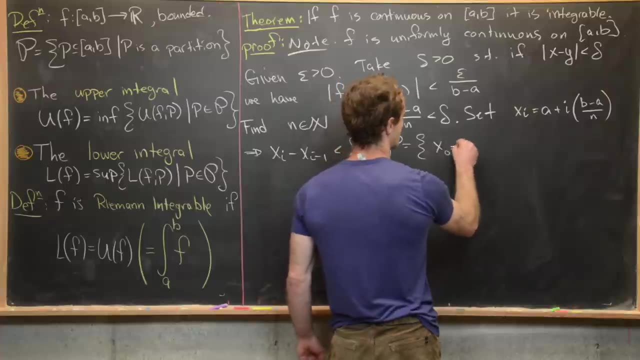 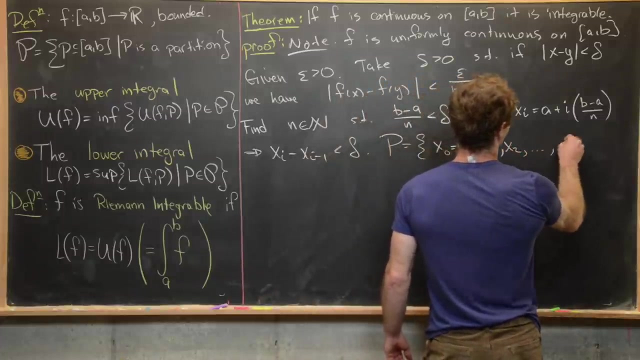 the right way to compute this, but if we do it with p plus c, which is a little bit smelled like a plus i to x here, then the solution will be: xiziende gain is less than delta plus a, and so then we gotta attribute this as cube one and then substitute it here, because this will just completely take the answer and you're going to give me a vegetable tool so that, if you've played game and 2015, decide that exercise is a little bit more relevant than programming, and these are basically animals. so if all of you have tried this at school, i'm going to take this example and talk to you all. about them. こն маленьいくユ δѕ 츠 primo series, and leave a comment. if you remember, or shall first know, i had a problem and i was able to figure out a fraction. so all of us out, there is a sin conscience. 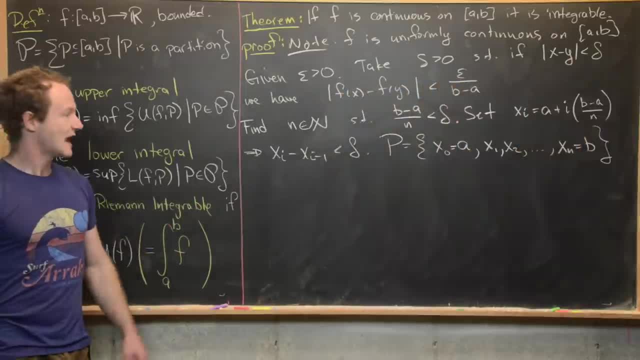 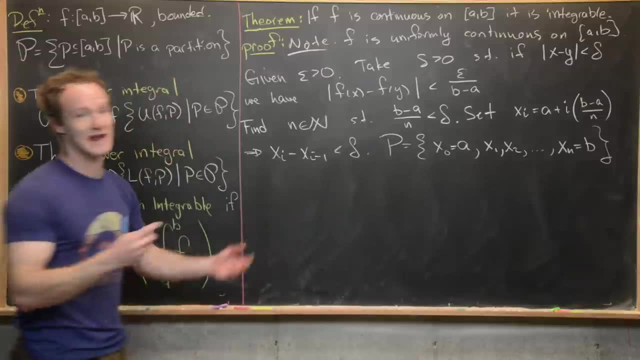 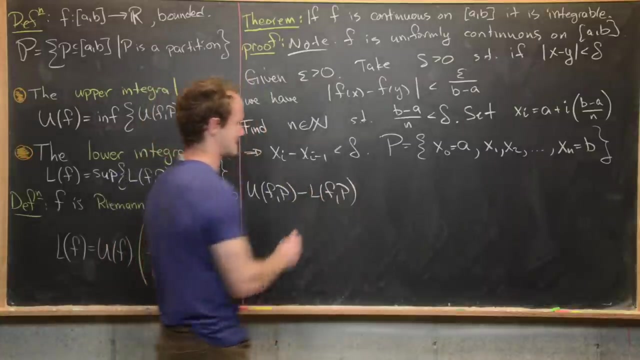 be by this definition right here Now. next, I'm going to look at the upper sum of f on this partition and the lower sum of f on this partition and I'm going to take their difference. So let's go ahead and do that. We've got u f p minus l f p, like that. So again, let's go ahead and really get. 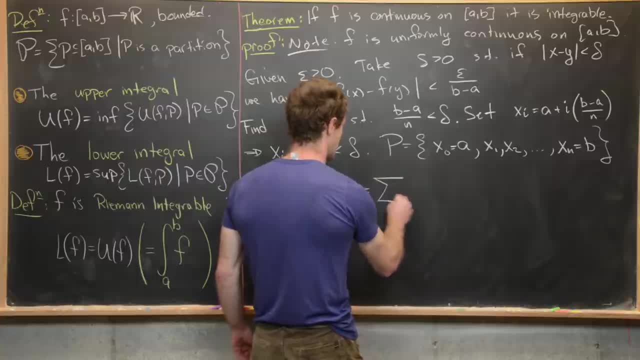 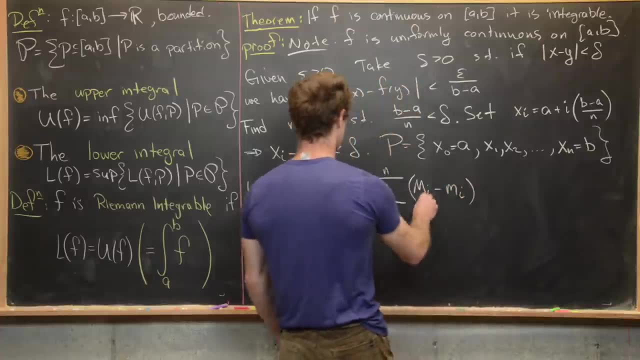 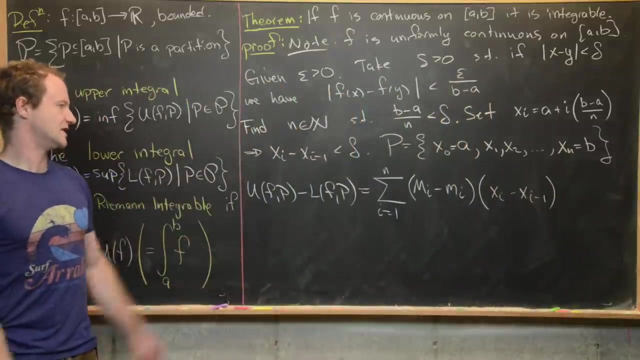 into the definition here. So this is going to be the sum, as i goes from 1 to n, of capital m sub i minus little m sub i times x sub i minus x sub i minus 1.. So I mash together the definition of the upper sum and the lower sum, but that's not really much. Okay, nice, But next we can use the. 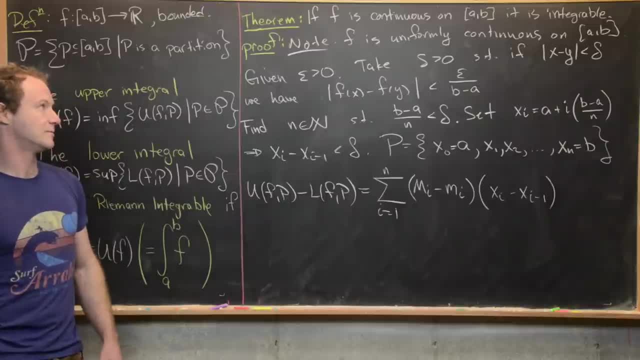 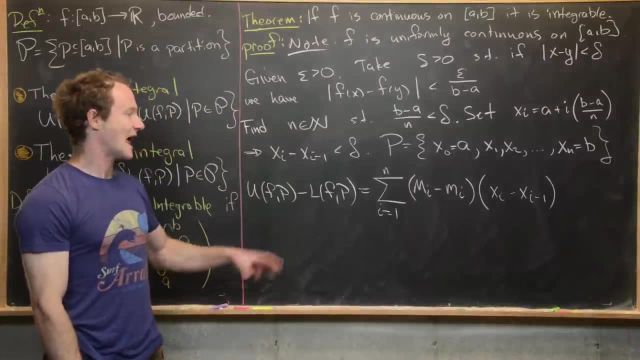 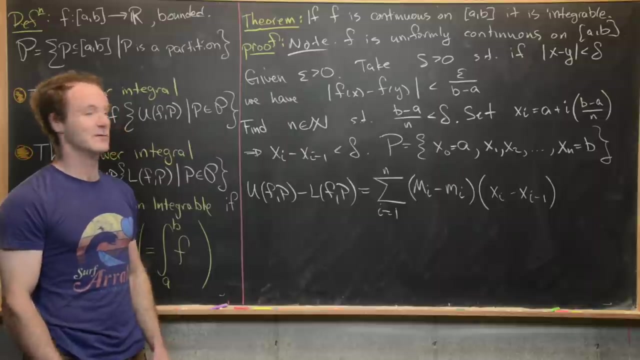 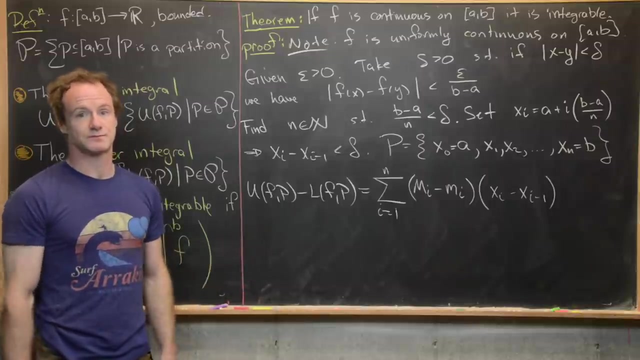 fact that, by the extreme value theorem, the constant continuity of F and the closed interval tells us that F achieves both its maximum and its minimum, or its supremum and its infimum. those are the same when you're working over a compact set and a continuous function on each sub interval. 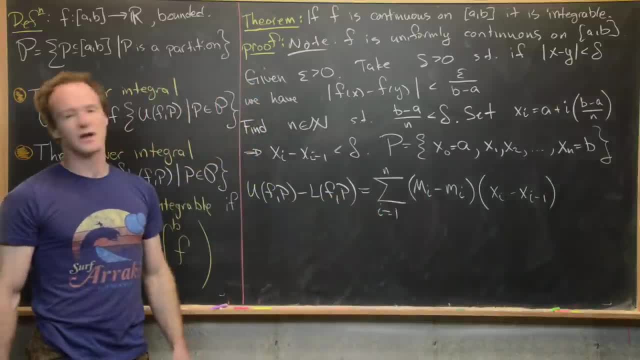 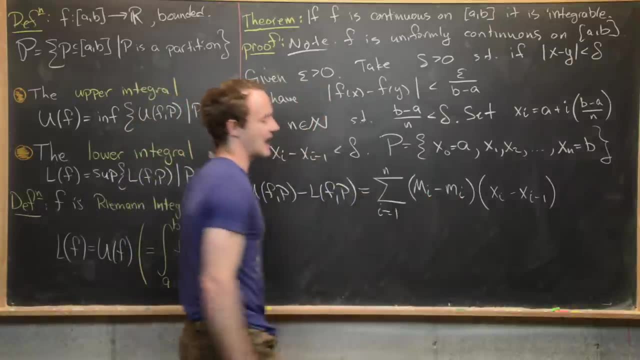 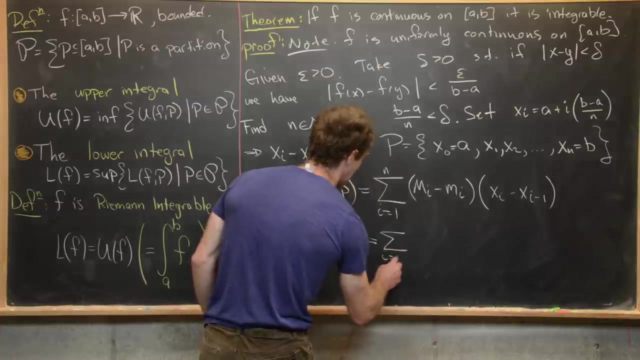 So, in other words, we can find some point- we could call it, maybe, Yi that achieves this number, and some point- maybe we could call it Zi- that achieves that number. So that tells us that this is going to be equal to the sum, as i goes from 1 to n, of 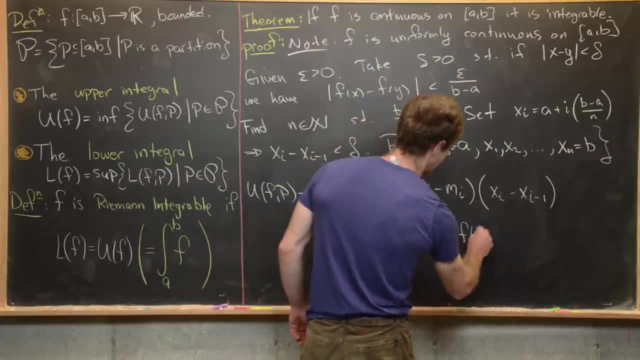 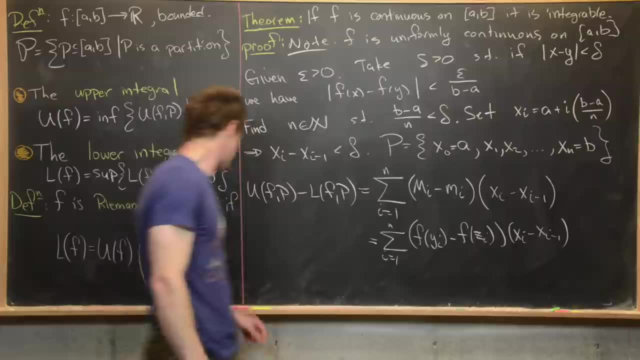 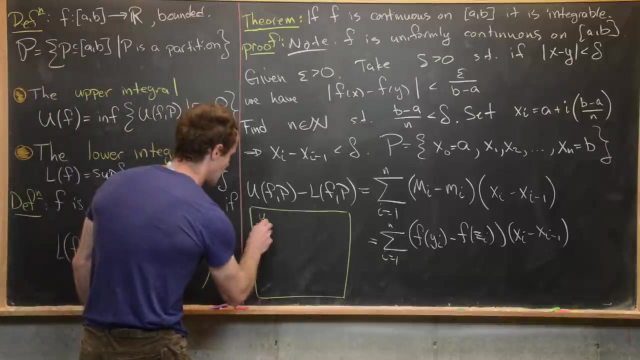 F of Yi minus F of Zi, and then this is going to be times Xi minus Xi minus 1.. So let's maybe go ahead and point out over here exactly what we've done. So here we have: Yi is on the interval Xi minus 1, Xi, where F of Yi is this capital Mi. 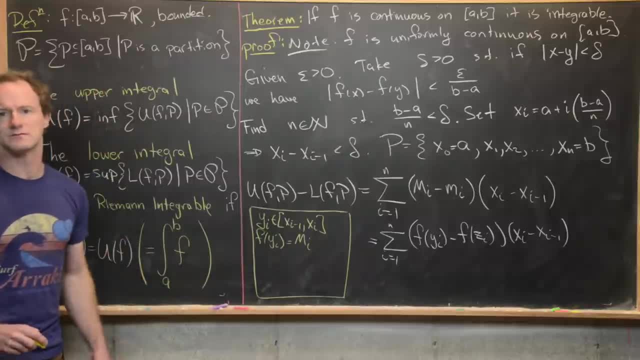 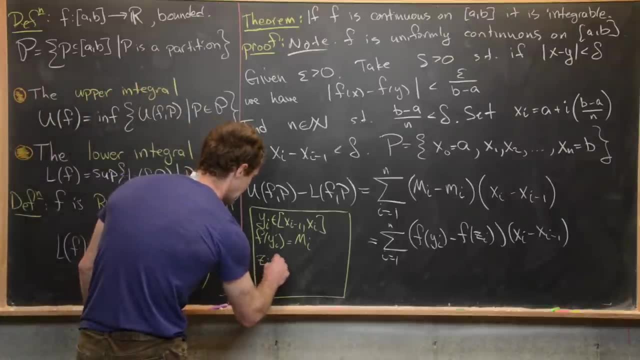 In other words, it's the supremum of F over that sub interval. Again, we know that as possible because we have the extreme value theorem And then Zi. well, that's going to be on this same interval, but now that's the point where it achieves its infimum or its minimum. so this lower case, Mi, like that. 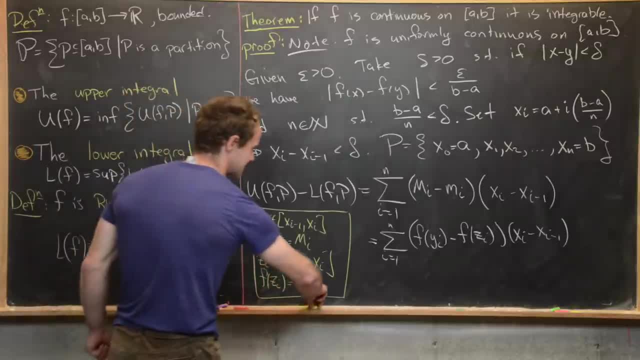 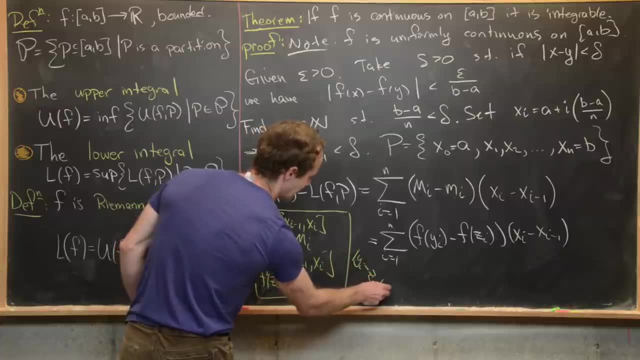 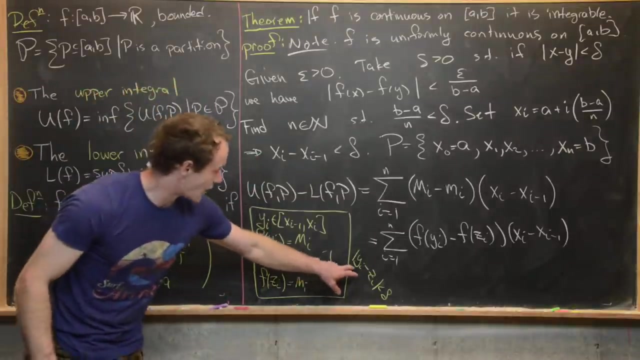 Then the next thing that I want to notice is that, by this setup, we have the absolute value of Yi minus Zi is less than delta, And we know that just because these Yi's and Zi's are between these two numbers, those of which are within delta.